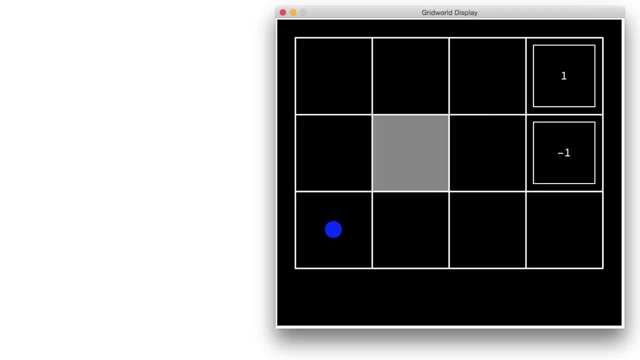 lot of time thinking about, or at least something very similar to this. So this is grid world. So in grid world we have, you know, a very simple board where we are. the blue dot, or rather the agent we're going to be thinking about, is the. 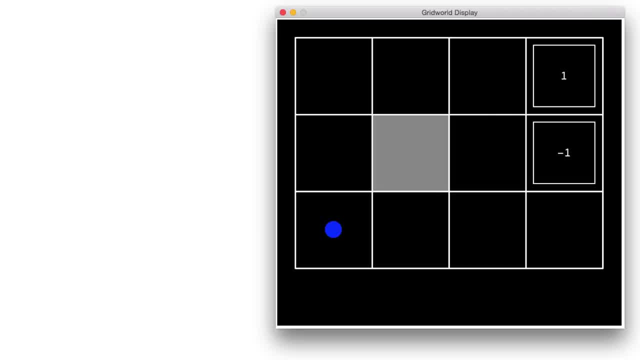 blue dot and and the agent is able to navigate through this grid. they can. it can move up down, left or right, and it has. there's a square that's colored in gray, which is one that the agent can't get through. that's a wall, that's an obstacle. and then there's two squares on. 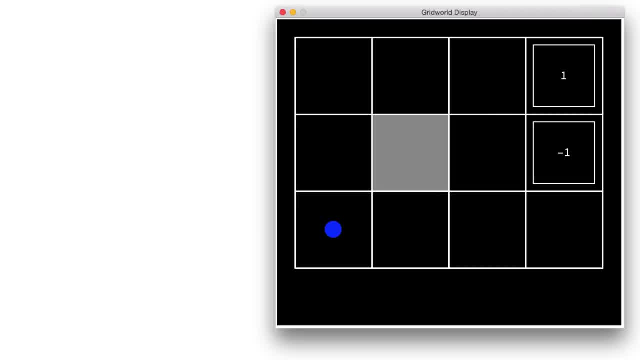 the top right that have numbers in them, and these states have reward values. in fact, one of them has a negative reward value, which is a penalty. so the agents goal is to collect this reward. so you know, naturally you can sort of look at this board, you know, and with our human intelligence we can think. well, you can. 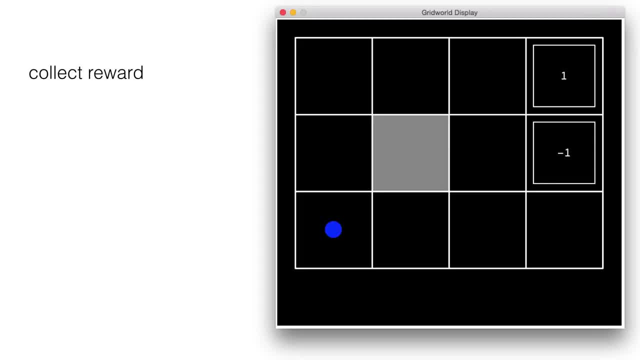 just search for that one. we can use our algorithms that we've studied so far to search for that one, the search for the path to get to that one, and that might be something like this: right, we take, you know, this simple path and the way that we used to represent things in search algorithms and maybe even in adversarial 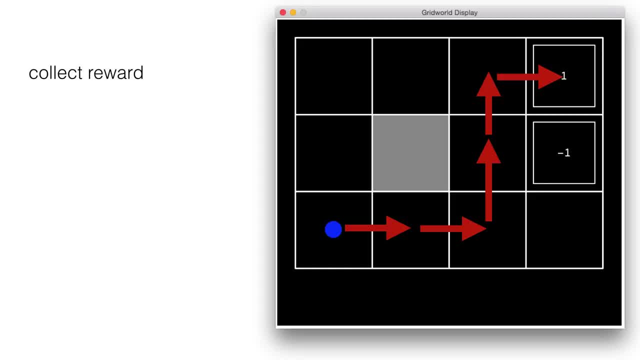 search algorithms. we've basically designed algorithms that return a sequence of actions right. in this case, the actions would be right, right up, up and right. okay, those are the directions of the arrows and those are the actions you take. that take you from the starting point, where the blue dot is now, to the 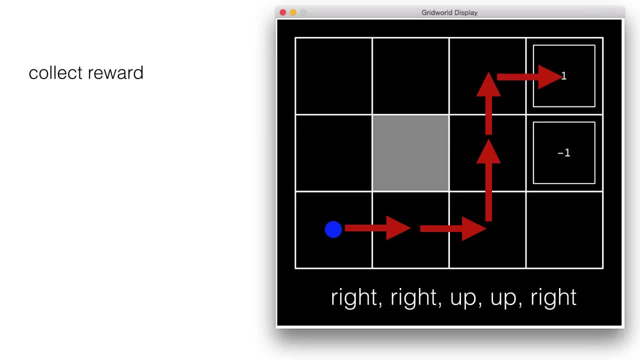 best goal, the best reward, which is one. okay. so the difference in the markov decision process representation is that actions don't always translate to state transitions, like right now in the search algorithms view and the minimax view or the adversarial search algorithms view. an action always leads to a state. 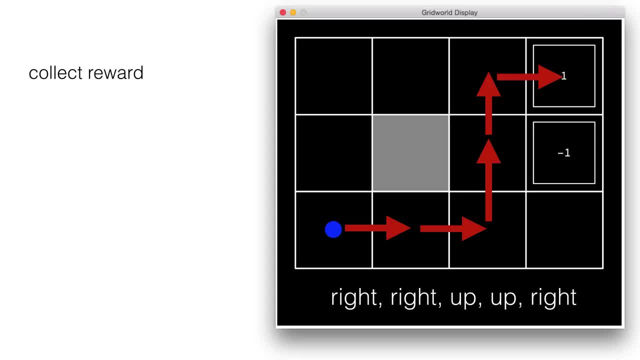 transition, it always leads to a particular transition to another node in our- you know- state space node, in our state space node, in our state space node network, whether it's a tree or graph, but in a markov decision process, actions are actions and state transitions are state transitions and they're not really. 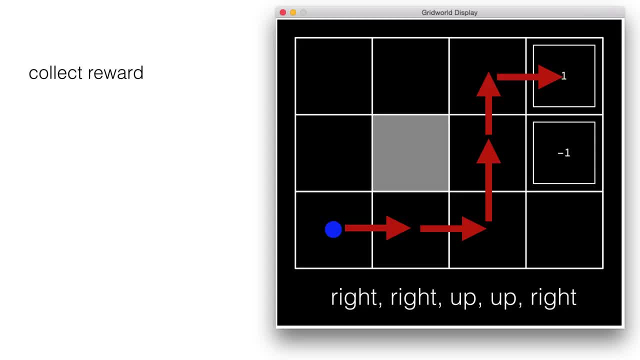 as inter, as intrinsically tied as they've been previously. so what we have with these stochastic transitions is that we might try to move right, we might take you know, choose the action right and something might go wrong. right instead of our robot moving to the right. if this is a robot, or its wheels might. 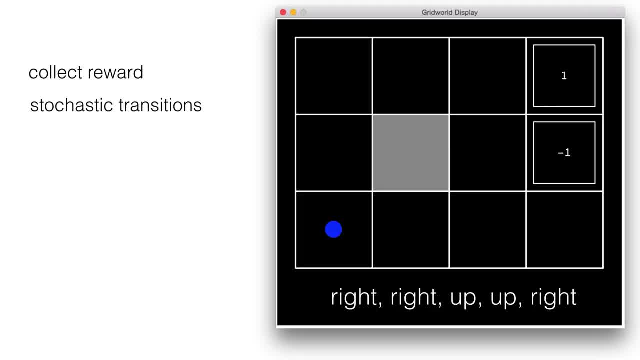 slip, or the terrain might, might give way and it might stay in place, it might move up, but you know, most of the time everything goes right and everything goes fine and our attempt to move right might succeed. maybe that's a nice optimistic scenario, but not all the time. and so this might look like this right if we tried to execute the same sequence. 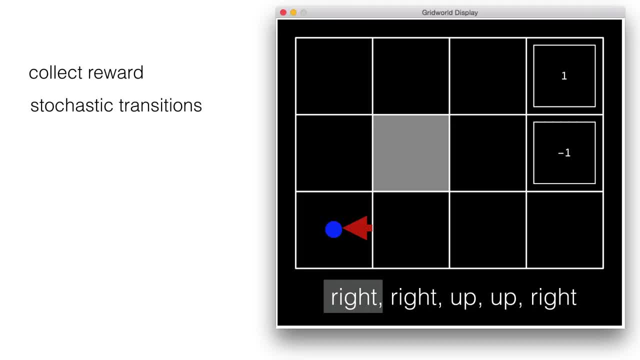 of actions of right, right up up right we might move, try to move right and fail. okay, we failed. and now we're: we didn't move, we didn't change state. now we try right again, continuing the actions that we've already laid out by our search algorithm. 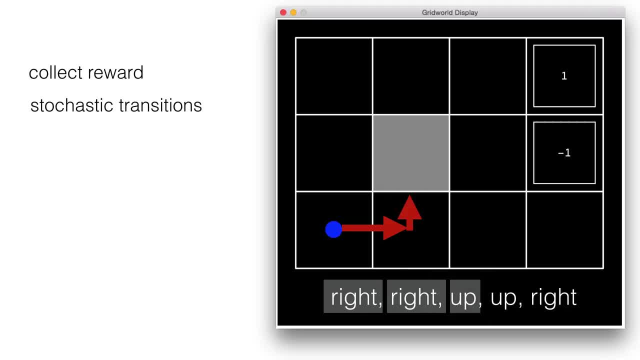 or by some other algorithm, and we try to move up, and that's illegal because it hits a wall. we try to move up again, it's a wall again. and then we move to the right and that's where we land, because we we memorize the sequence of actions. 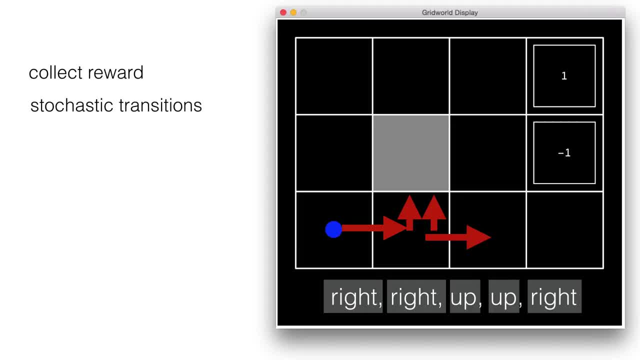 we were not robust to the fact that the the environment might not allow us to make the actions that we want or make the transitions that we want. we can take the actions, but the transitions might not happen the way we expect them to, or, you know, worse. another example of this could be: you know, we successfully move right, we. 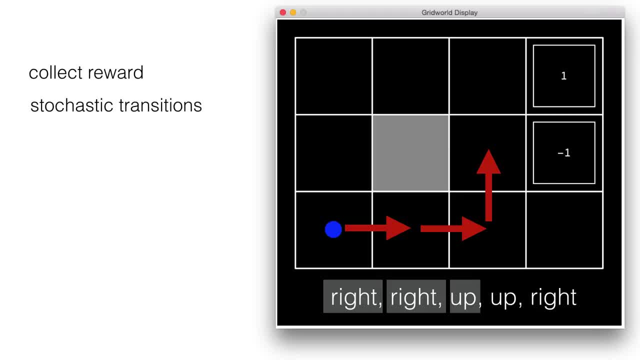 successfully move right, then we successfully move up, and then, for some reason, our wheels slip. we try to move up and we slip, and then we move right with the final move and end up on the minus one square. so not only did we get no reward like we did in the first, 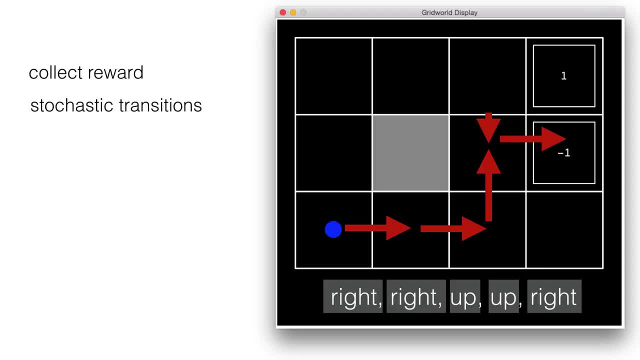 example, we actually got the worst reward. we got the, you know, got the penalty. okay, so in order to handle this type of environment, or this just twist on what environments can be, we're gonna want to represent these things formally. so how do we do that? so we have a probability distribution over. 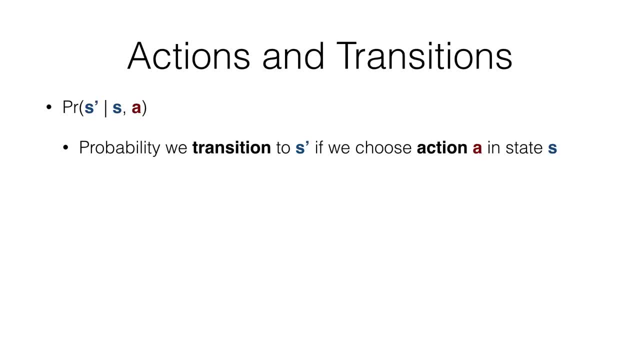 what state we end up in, given the current state that we're in and the action that we choose. okay, so think about this way: if we're in, you know a square, and we choose the action up, we choose the action to move up, then there's some probability that's supposedly going to co-exist with some aging. you know well, there's some probability we're going to end up. 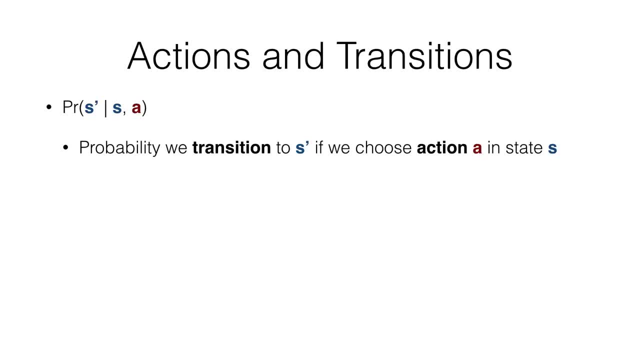 in the square above. there's some probability maybe we'll end up in the same square and maybe there's some probability we end up to the right or left. but but this function, this probability function, is something that is part of the the environment description. right, it's part of the way. 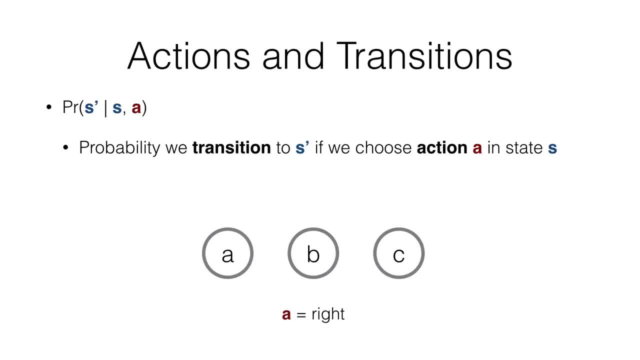 we represent the environment. so an example of this is illustrated right here with these three states. so there's a being states a, B and C, and let's say we're in state B, okay, and the action we choose is right. so normally this would be the whole story right, if we choose right or not normally, but at least in. 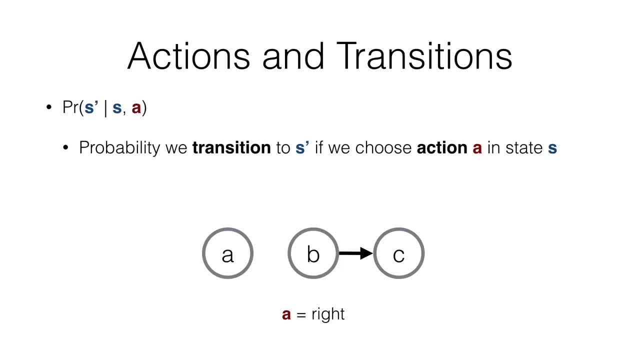 the things we've been studying so far. if we choose the right action, we're gonna end up in C. that was the old way of thinking. right now we're gonna say, okay, well, if we choose right, you know a equals right action, equals move right. maybe we'll accidentally stay in the same place or maybe we'll move to the 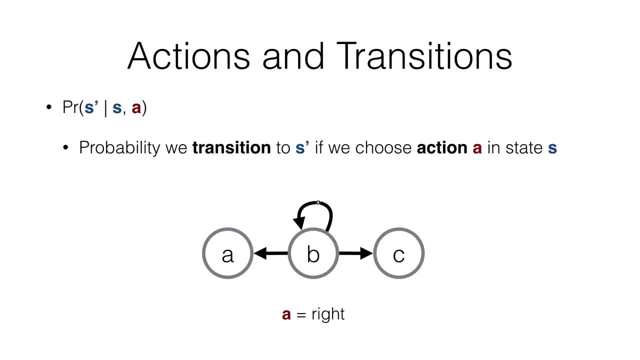 left, like I said. and then here's you where the values of these probabilities might come in. maybe the probability we successfully move to the right is 0.7, and the probability that we slip and stay in the same place is 0.2, and the probability that we backslide maybe is. 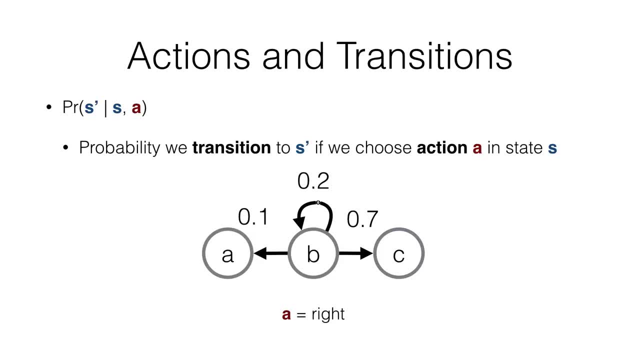 0.1.. And so these sum to 1 form a valid probability distribution. you can think of it as just a fraction of time over all the trials that you're going to ever try this action from this state. what's the fraction of those trials? 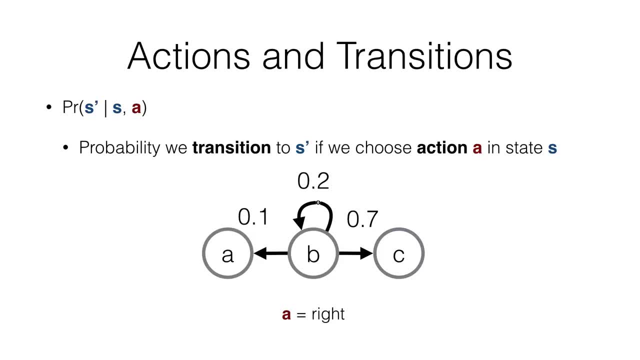 that you end up in the subsequent states- in C, B or A. And the other thing to note is that this is a strict generalization of what we've seen previously, So you could imagine having a probability distribution like this, where it's a 1.0 that you end up in C. 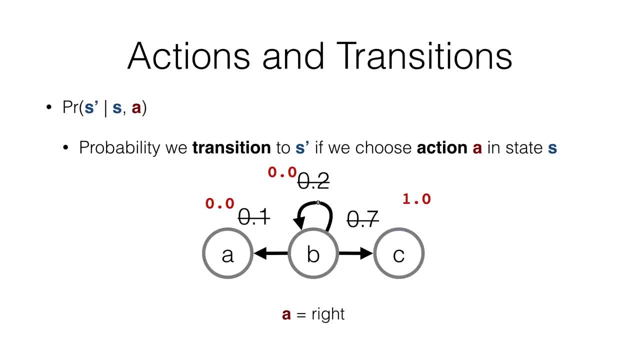 and 0 that you end up in the same state and 0 that you end up at A, And that would be- we'd call it- a deterministic Markov decision process, which is pretty much what we've had previously, where we just had a function that returns. 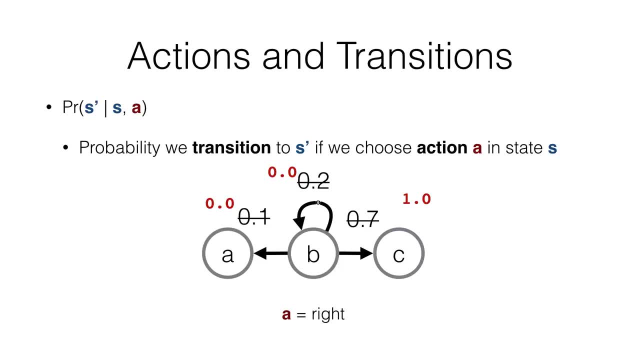 the next state given an action. And here I've written out how you map from these numbers I threw on the screen and these pictures I drew to the probability function. So the probability all the way on the right, the probability of state C, given that you're starting in B and you take the action right. 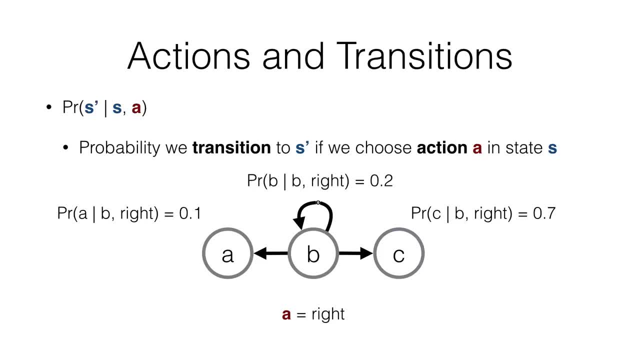 is 0.7. and then the probability of you're in B, given that you were in state B and that you take the action right, is 0.2.. And the probability that you end up in A, given that you were started in B and took the action right. 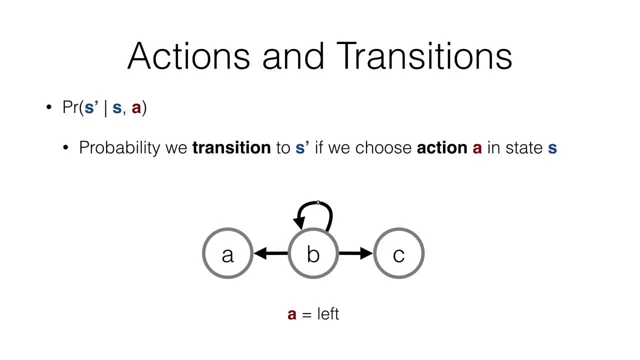 is 0.1.. So now suppose we move to the left and suppose when we try to run the same, when we try to move to the left, we get these probability distributions or this probability distribution, And maybe this basically implies that moving left is slightly more successful. 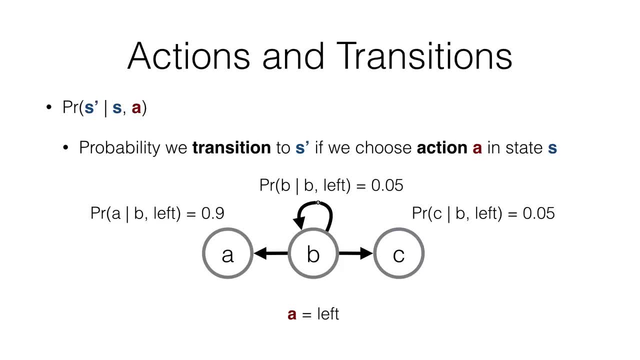 than moving right. Maybe this could be something in the terrain again, or it could be something about the nature of transitioning from states, But the idea is that we've written out completely different numbers, completely different probability distribution for a different action, So you can. 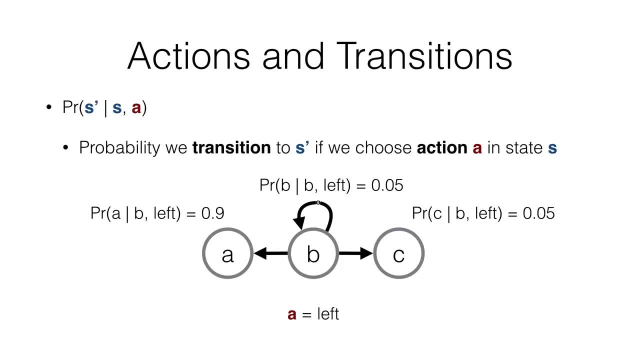 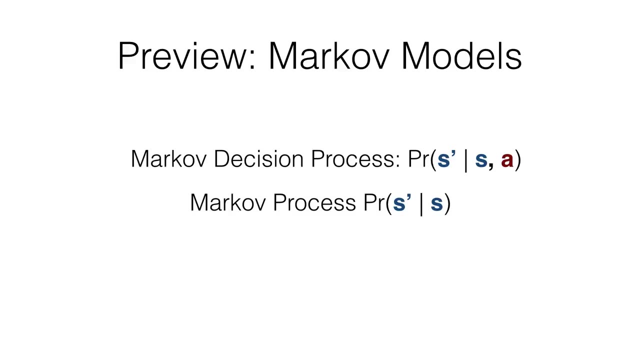 just plug in whatever action that is available for you from state B and then you get the probability distribution back. Or when we design these processes, we have to consider all the actions from every state. Okay, And as an aside, you might have heard about Markov models maybe. 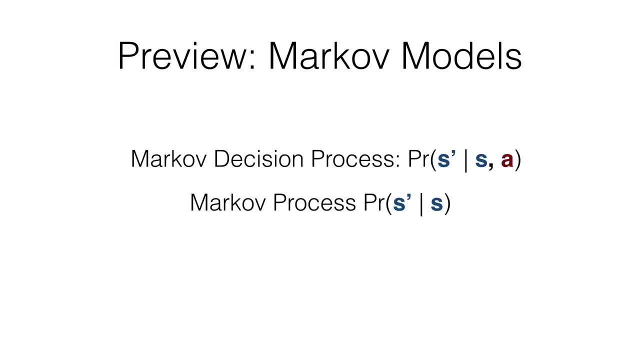 in other classes. maybe if you took Econ or some probability or some stats classes teach these things. Or maybe if you're in the math class, you might have heard about Markov models. And maybe if you're in the math class, you might have heard about Markov models. And maybe, if you're 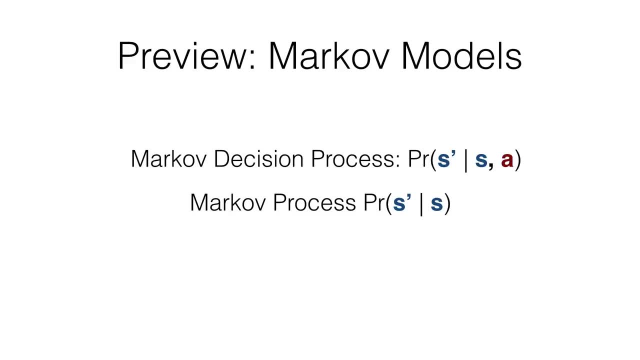 learning, machine learning- you might have learned about these. So there are these things called Markov models, which are kind of a simpler version of the Markov decision process. Basically, a Markov process is where you don't have the actions right, So you don't have a decision. 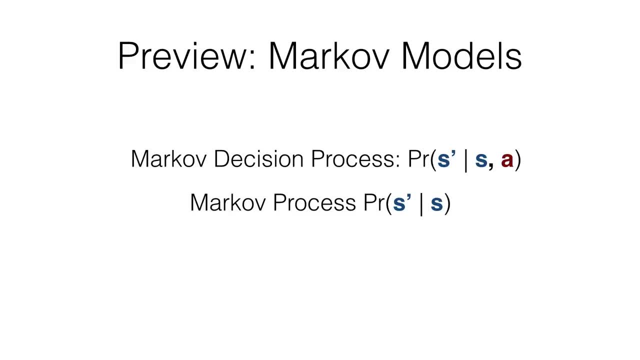 to make. So that's an easy explanation for why the things are named the way they are right: Markov decision process versus Markov process. So in a Markov process you don't have a decision to make. All you have is a bunch of states and a bunch of probabilities of 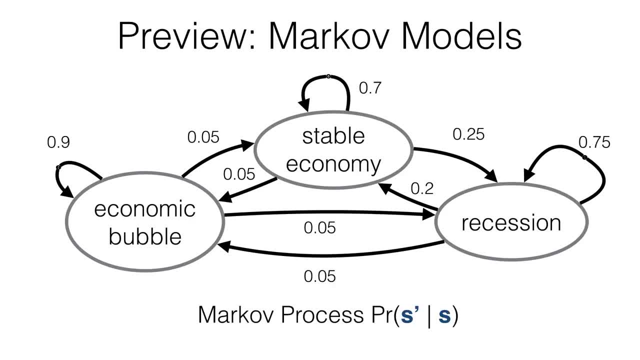 transitioning between states, And people use these things to model, you know, transitions between modes of like the economy, right? So here's an example. Try not to show this to any economics professors. they'll be really mad that I'm really misrepresenting what actually happens. 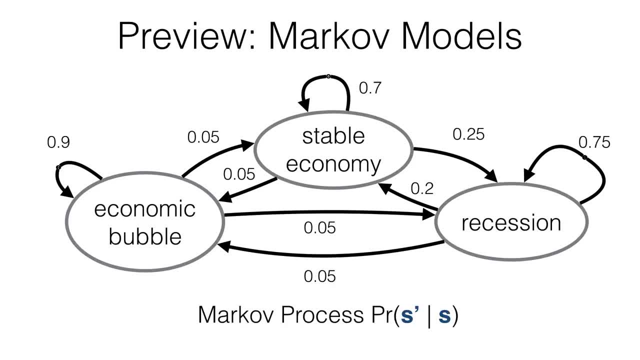 in real economies. But you know, here's one, maybe plausible model for how things behave in economies. So maybe you have economic bubbles and if you're in a bubble you have a 0.9 probability of staying in that bubble. 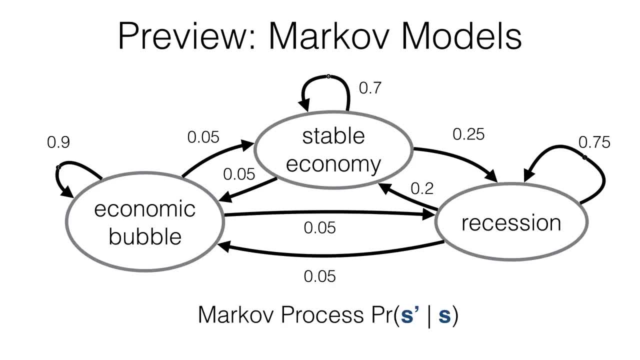 But then every now and then you know 0.05 of the time you move from the bubble to a stable economy And 0.5 of the time, 0.05 of the time- you move from the economic bubble to a burst. 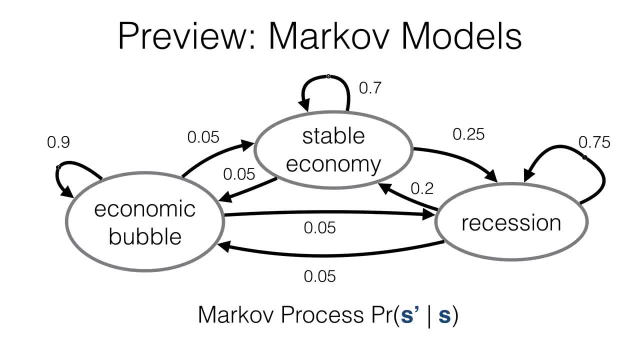 and you get a recession, And then maybe a recession stays in a recession or stays a recession 0.75 of the time, and sometimes it transitions to the stable economy, et cetera, et cetera. Let's not think too much about this, But the important thing to note. 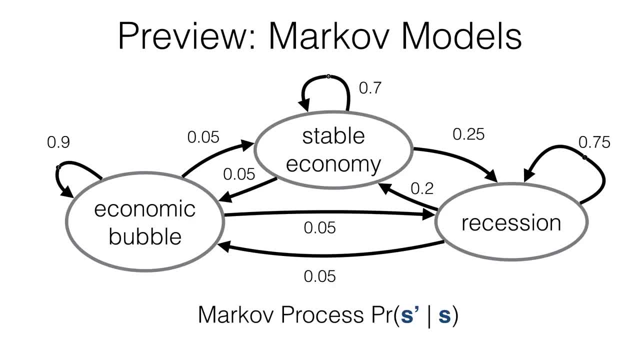 is that in a Markov process, there are no actions, right, So it's just the transitions. it's like thinking of a Markov decision process where there's only one decision, there's only one option in every state, which is just to move on to the next time step. 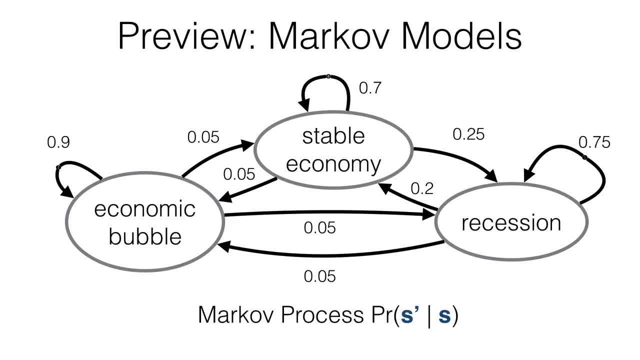 So a Markov decision process gives us a little bit more agency, you know, which is very fitting, right? So it allows us to task our AI algorithms with a decision to make at each time, step, at each state that you're in. 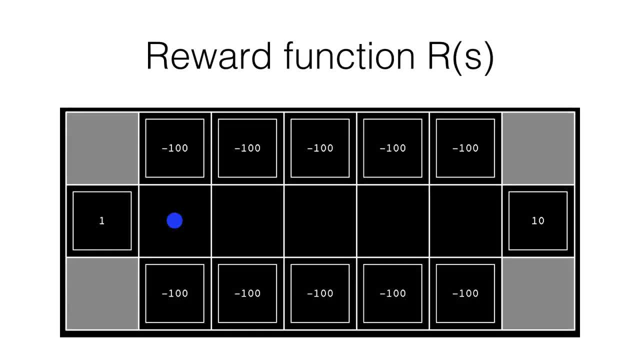 back to Markov decision processes. let's think about the reward function. So we saw this very simple grid world with a reward function of a 1 and a reward function of a minus 1, which is the penalty. So this is the bridge, the slippery bridge variant of grid world, And the idea is that you 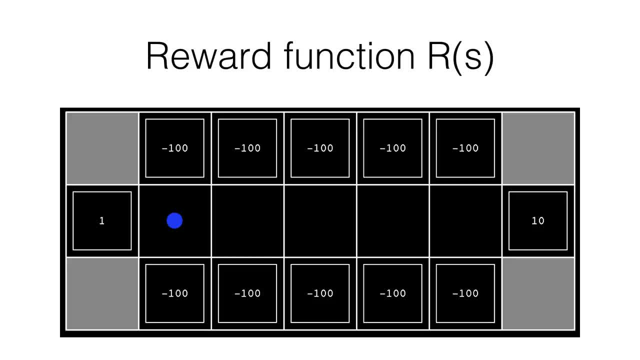 are at the blue dot and you can see that there's a reward square on the left. You can get one reward- a reward of 1, if you move to the left, But if you move to the right all the way across. 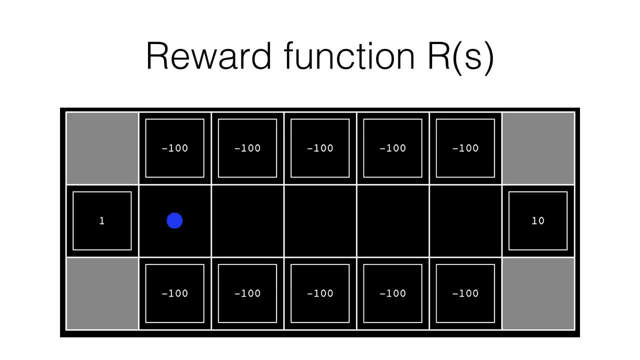 the bridge, all the way to the right, there's a 10. And then, along the way, adjacent to this path of zero reward, there are these minus 100 squares. These are the penalty squares, And what this is meant to represent is a situation where a robot is on a bridge. The bridge is all the empty squares. 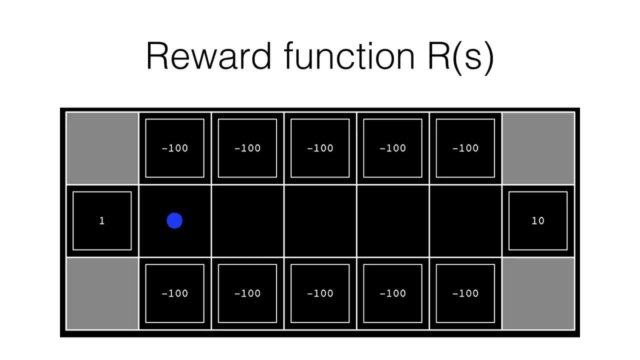 with zero reward And the across the bridge there's a pot of gold That's a 10.. So you're really going for that. Or if you really want to get the highest reward, you go for that 10.. But the problem is, the bridge is. 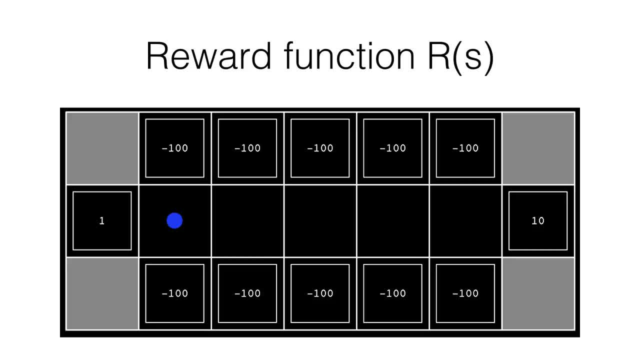 slippery. So when you try to move right on the bridge, maybe you'll slip off the bridge and fall down into a chasm, and that's worth 100 or minus 100, right. So you get penalized hugely if you fall off. And so the question is: you know this is, I guess, a representation of many problems we. 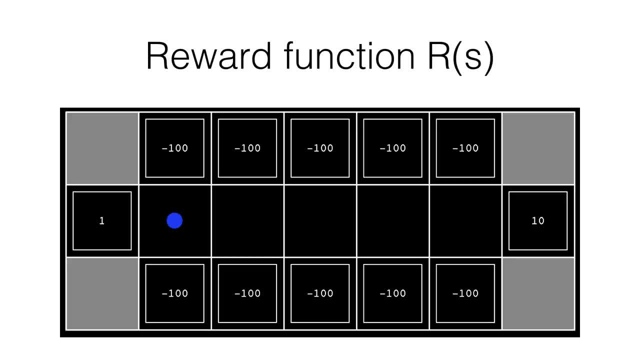 have of risk-reward in real life is: do we risk crossing the bridge to get the 10 reward or do we just take the one reward? you know, take the safe way. So the way we answer questions like that of you know what do we do in this. 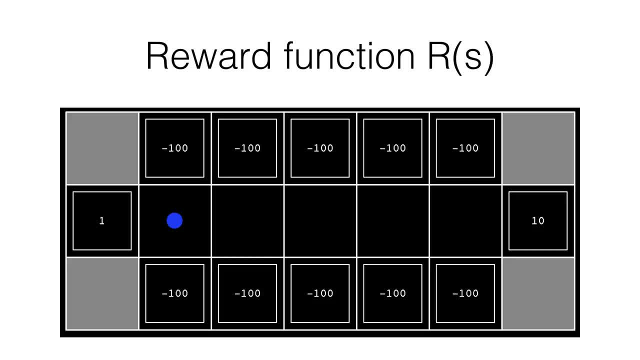 environment. And what do we? you know, how do we get a good reward in this environment is we propose a policy. So we try to come up with a policy which is a function- or formally you can think of it as a function- of the states. that just tells you what action you're going to take, And so 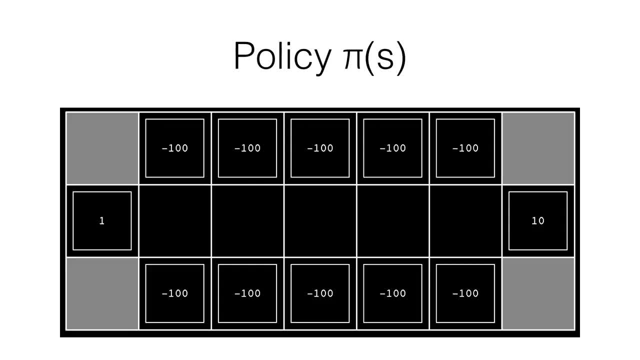 what you're going to do is you're going to have a policy that tells you what action to take in any state. okay, And this is richer. this is much richer than a sequence of actions, right? Whereas before we saw that example where, if we just write down a sequence of actions, if your transition 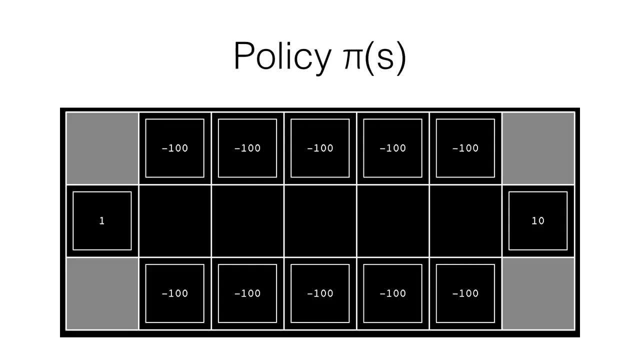 takes you someplace you didn't expect to be. you don't know what to do anymore if you just have a sequence of actions. But now, if you have a policy, then the policy. you can always evaluate it into this, in this new state that you accidentally found yourself in, and it will tell you what to do next. 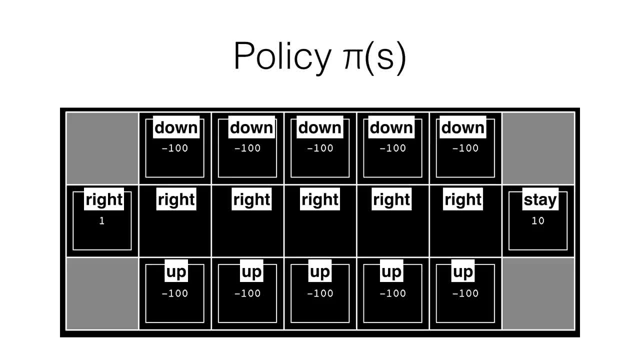 and what action you should try to take. And so here's an example of one possible policy that you could, you know that you could consider in this bridge, slippery bridge world, right, So you can see that you know I did this by hand, so you might get, you might see where I'm, how I'm thinking. 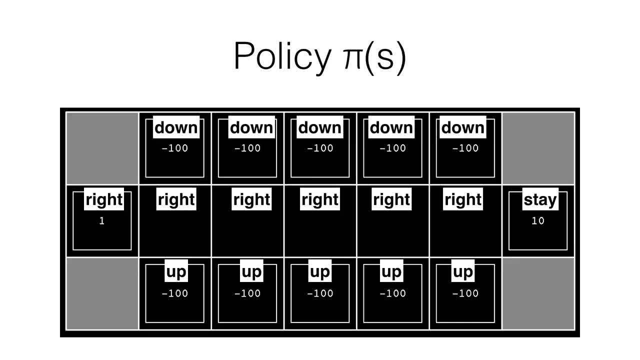 about this I'm. it's basically a very greedy policy. The greedy policy tries as hard as it can to get to that 10. And even if it's, even if it's in the one spot, even if it's in that safe reward spot all the way. 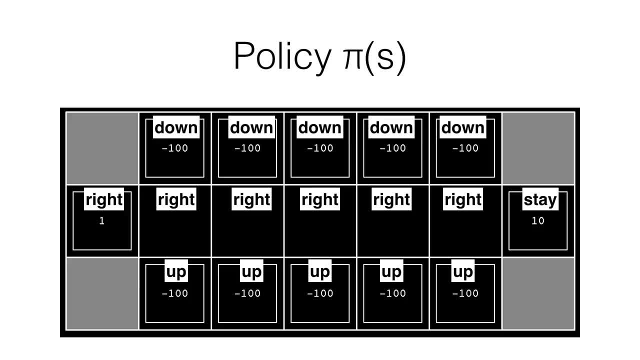 on the left, it's going to still keep moving right and try to try to get to the 10.. And then, if it falls into the chasm, if it falls off the bridge, it tries to get back on the bridge. So so here's. 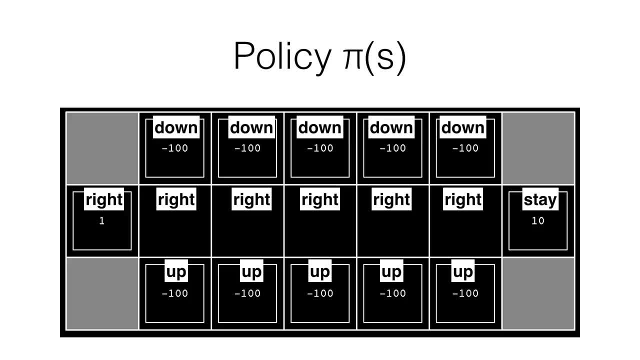 a question: Is this a good strategy? Is this, how do you know if it's a good strategy? The answer to that is: is that you actually, you don't know. We don't know if it's a good strategy because we. 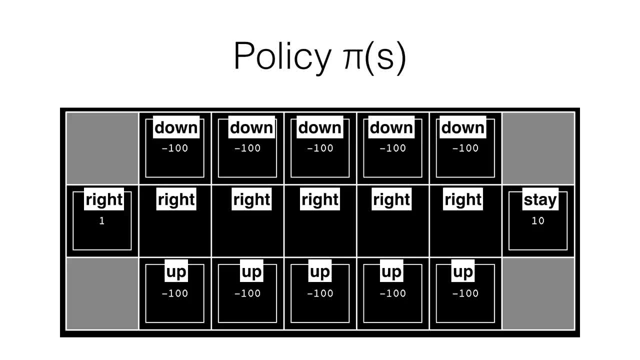 don't know the transition probabilities In this graphical representation, where all I've shown you is a grid of states, of states, there's, there's nothing on the, on the on the page, right now, on the screen, that really tells you what the transition probabilities are. 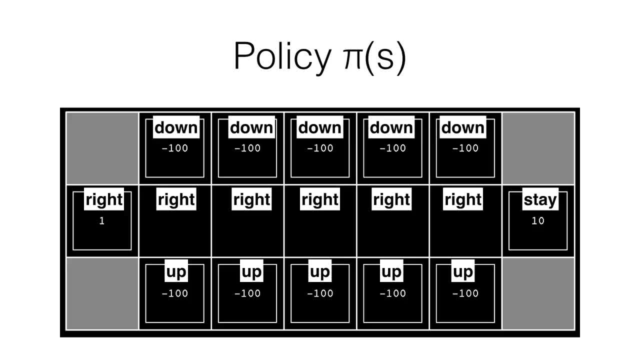 You know? for, for example, you could imagine, you could imagine a situation where this strategy might be, or this policy might be, a better one, right? So, in this policy, if you're on the bridge but you haven't gone far enough, maybe you want to move left and stay, and 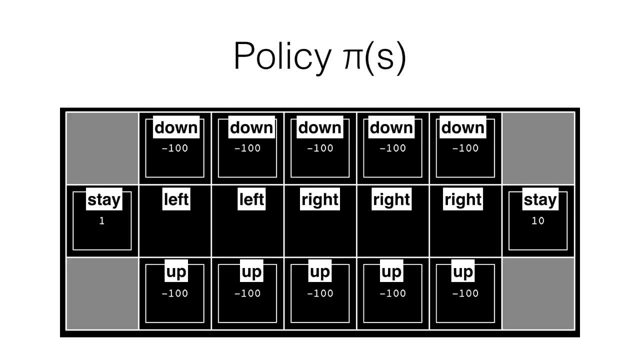 get that one reward and be safe instead of risking crossing the entire bridge. I don't know. It depends on. it depends on the, the transition probabilities. So even if if we have these transition probabilities, then we want to ask ourselves: how do we measure how good a policy is? 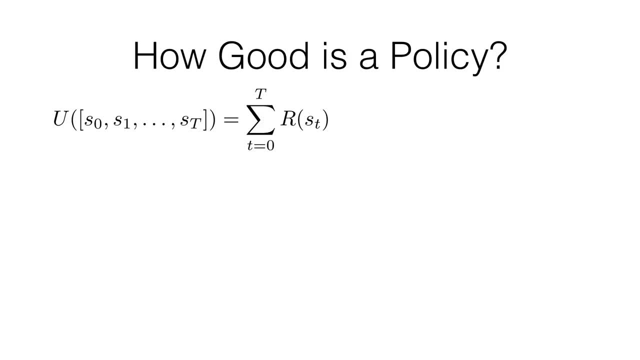 So so here's one way to do it. We're going to use use the function U to represent the utility of a sequence of states. Okay, I mean, this is pretty kind of obvious, an obvious way to do it. So. so what we're going to do is we're going to say the 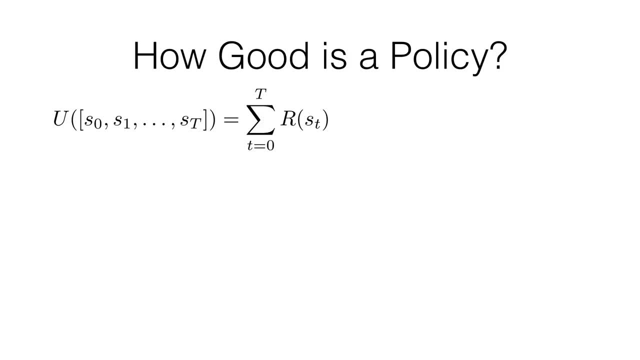 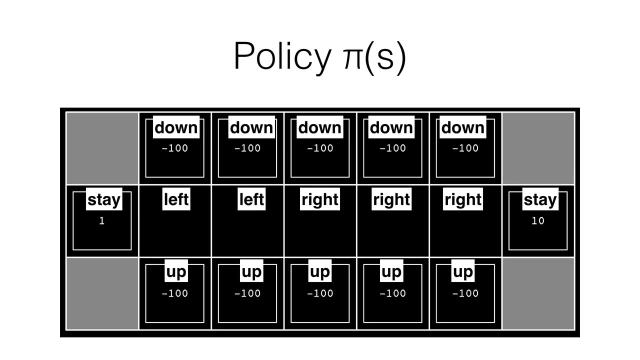 utility of a sequence of states is the sum of all their reward values. And in you know, in the this grid world thing, most you know, many of the states have zero reward. And when it's when it's zero reward, I didn't. these diagrams usually don't write the actual. 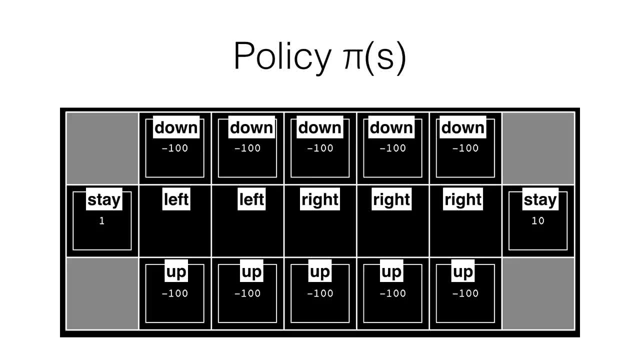 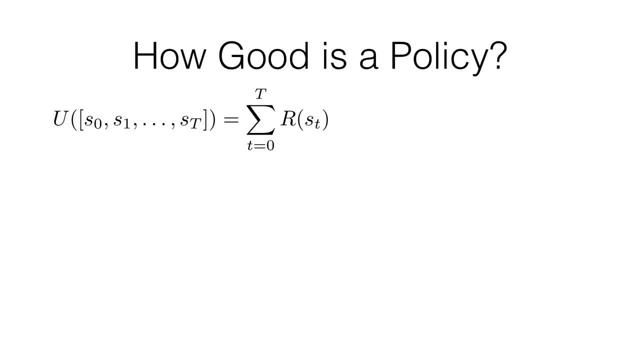 the reward value on the screen Just to eliminate clutter, but most of the time that's zero reward, but that's okay. The point is that for every state in the sequence you have some reward value and you're just going to sum them up And that's fine, That that that's a reasonable way to start. One of the problems is: 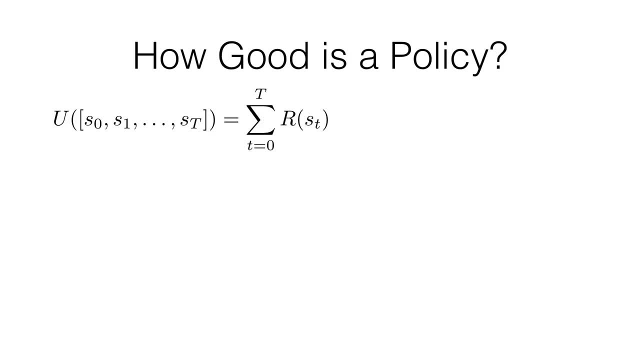 that you know. what I've written here is that the sequence of states that you reach goes to, you know, from zero to T. So there's T states in the sequence. In many settings we want to consider agents that operate indefinitely, right, So so they operate forever. They, they say they just. 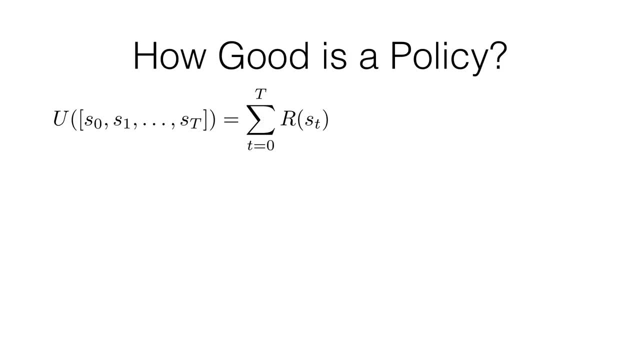 run around in the, in the environment, and try to collect rewards- and they are, you know, they're just rewarded for for living in the good states and avoiding the bad states. So if you want to have a function that evaluates the quality of a sequence of, you know, infinite states- because 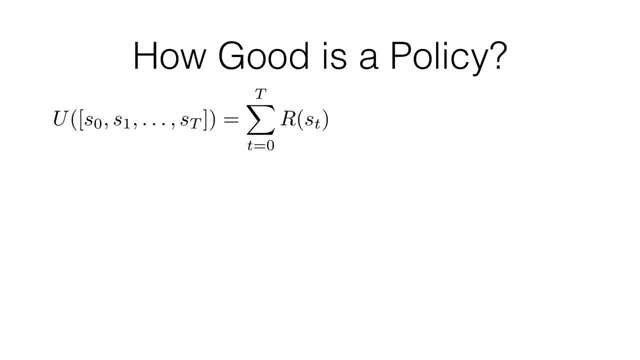 time in this scenario would go on forever and the agent would live in the environment forever. that value is is going to be very easy to end up being infinite And then, and then it's very hard to make a decision about what's a better policy. So one strategy for handling this: 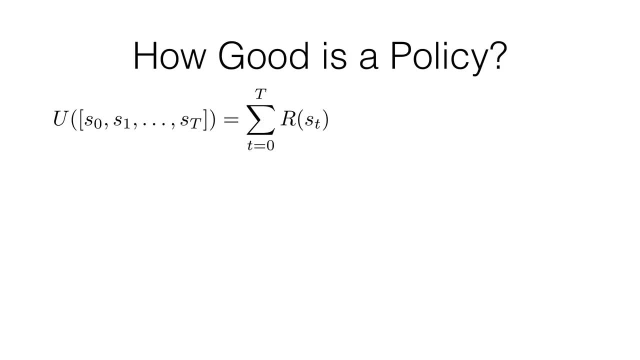 which is the strategy we're going to pretty much use throughout the rest of the, the segments of the course, is to use a discounted reward. Okay, And what? what this is is a. you put a number in front of you know, you multiply each reward by some number. that that's a sequence according to. 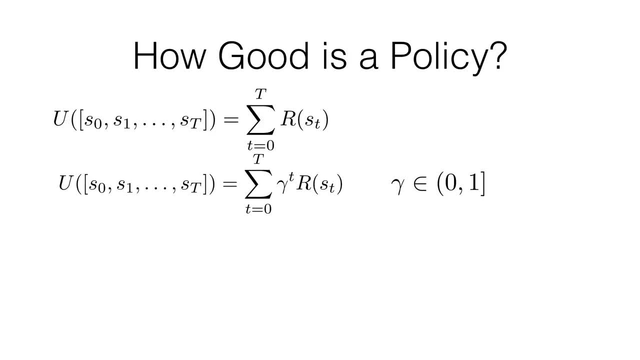 um the. you know how far in the future we're talking. So state zero, S zero is the current state, S one is the next state, S two is the state after that. So so S T is T steps in the future. 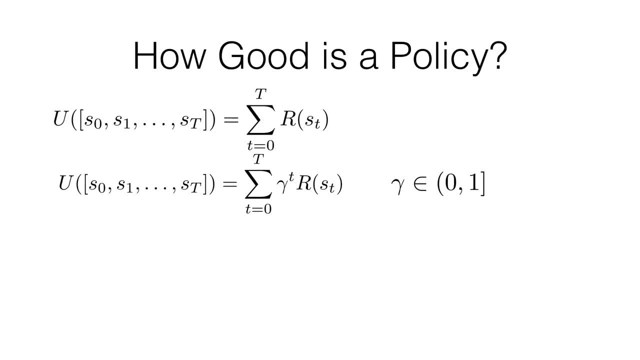 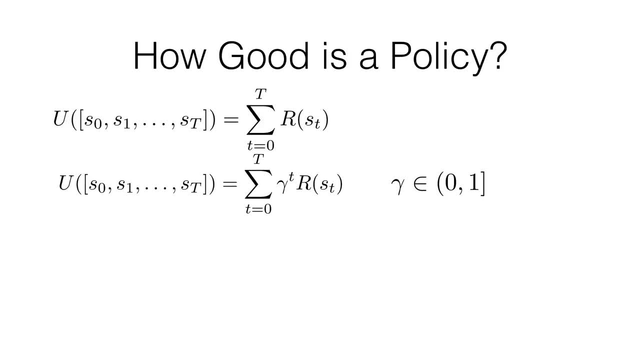 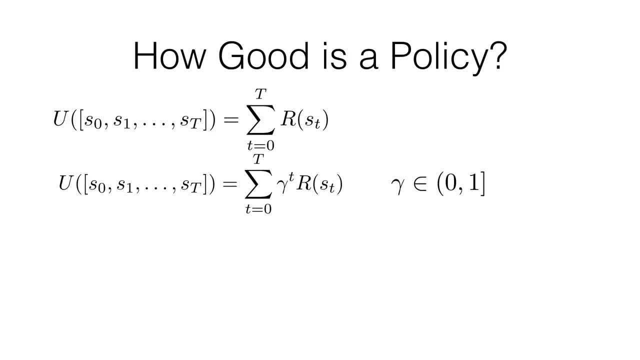 amount of influence you get, uh or amount of reward you're going to consider in the future. So if this is zero, then all you care about is the next state, uh reward. But if this is one, then you care about, you know all the reward forever. But if it's something in between the 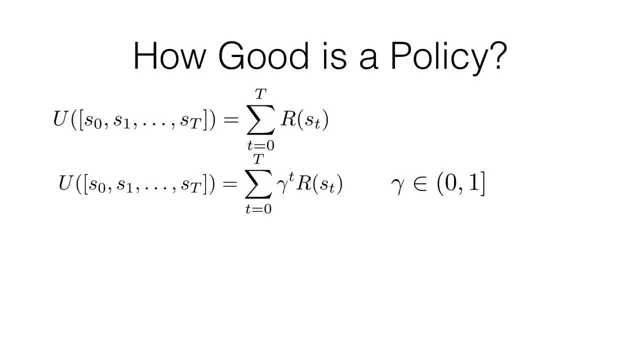 numbers, then you get that. you will, you know, slowly decay how much you care about future rewards. Okay, so so far what we've seen is just a function that takes in a sequence of states and tells you how much reward you get. 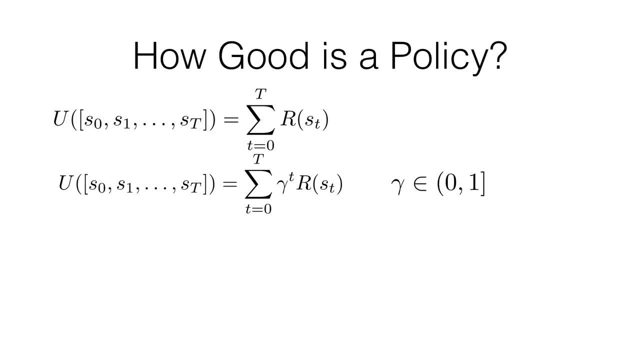 And that's not super helpful right now, or at least it hasn't gotten us very far, because what we want to evaluate, what we want to think about, is a policy. and given a policy, how good is it? And all we have now is just a defined way. 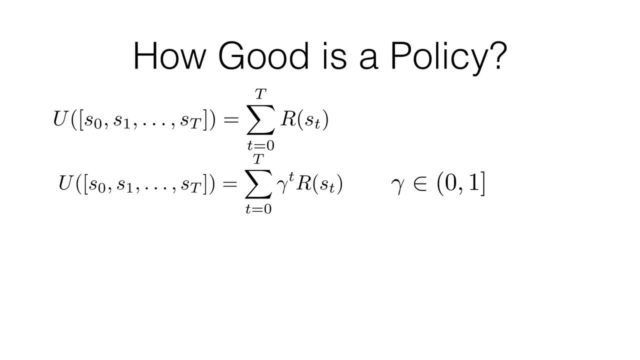 of thinking about a sequence of states and the reward you get for that sequence. So let's take this a little bit further. So the first thing I want to do is just- I've already hinted at this, but let's just say this sequence goes on forever. 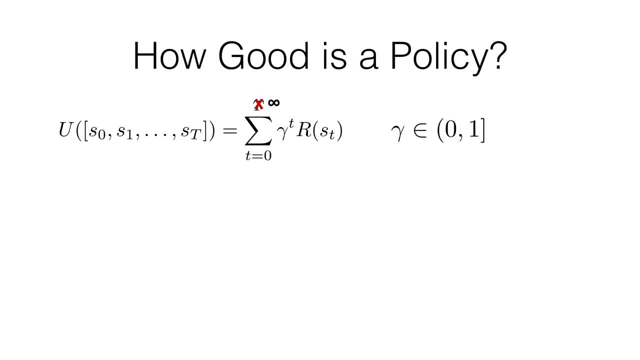 So it goes on to infinity. So, instead of to T, instead of to capital T, it goes to infinity, and the sequence is infinitely long. Or equivalently, T equals infinity, Capital T is equal to infinity. So now what we're going to do. 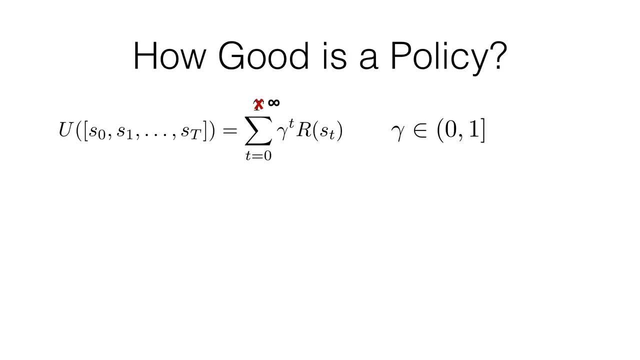 is we're going to write a more general utility function for states and policies. So this is U with a superscript of pi of S. So if you're starting from state S, what this says in English, just forget about the math for now. 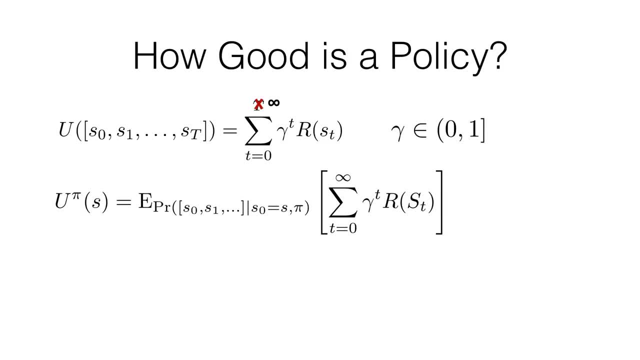 in English it says: if you start from state S, what is the expected utility of all the sequences you could see from starting from state S? And that's what that little probability in the subscript is And what this? what the math says is the expected value. 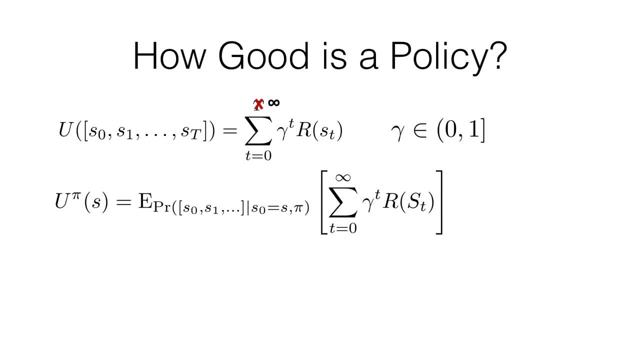 over the probability of all state sequences, of that state sequence score. that's above upstairs. And given that, right now, this is a function, now this is a function of a policy and of a start state, And so then, if we know what the initial state is, 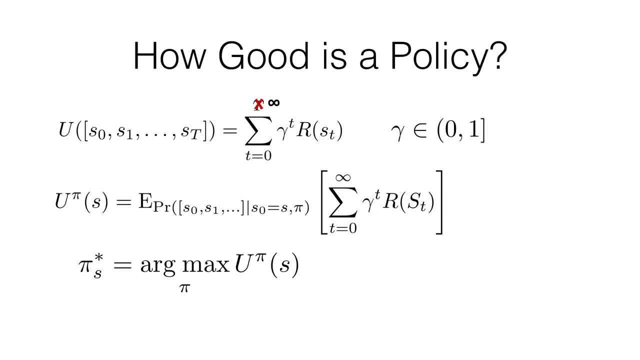 what S is. then we can just say: okay, here's the function we want to maximize, Here's what we, here's how we decide. what is the best policy for us And the best policy for us, starting from state S. 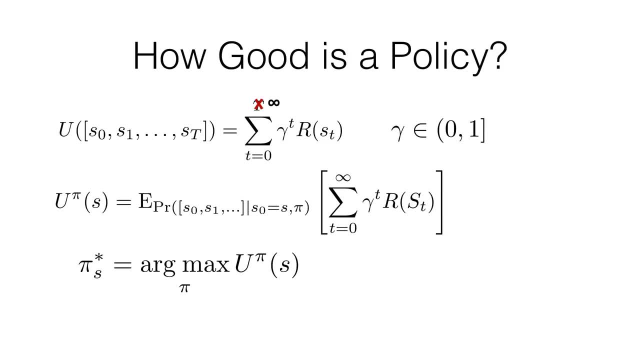 is the policy that gives us the highest expected reward for over the probability distribution of all sequences that we can get, starting from state S. So that's fine, that sounds fine, but what's weird about this is that we actually have now- have you know- a definition of a optimal policy. 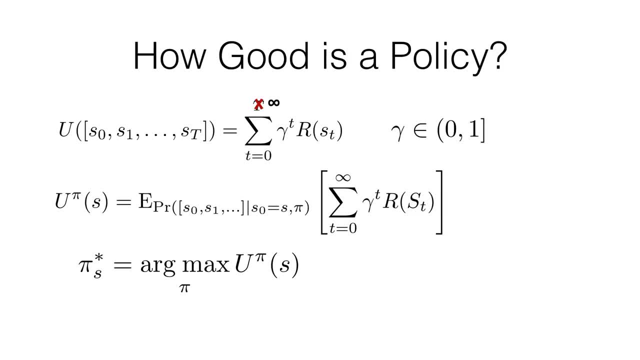 for every single possible initial state And that's kind of weird. but the good news is that things actually simplify a bit And the textbook gives a really nice intuition as to why this simplification works, And the idea is that you know, it's written down here. 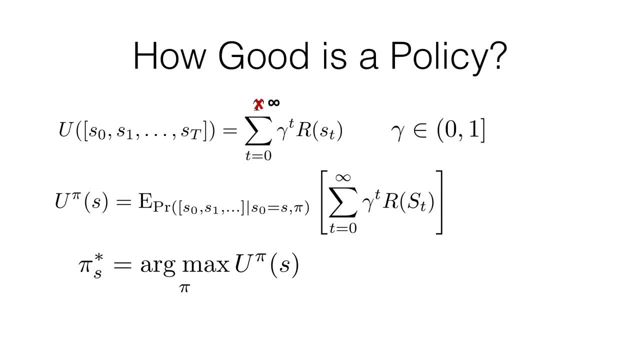 with this within math. if you work through the equations, it says that this is the expected or this is the score starting from state S And the score is for a policy that will consider, that will tell you what to do in any state. 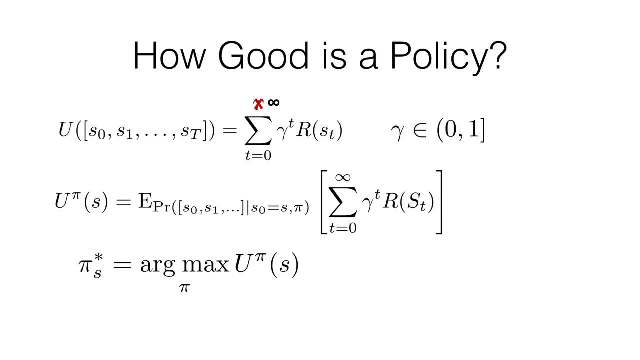 It will tell you what to do. you know, no matter what state you end up in Right. And the point is that if you imagine a different, you know a different policy, a policy starting from a different state, that also has to have you know actions. 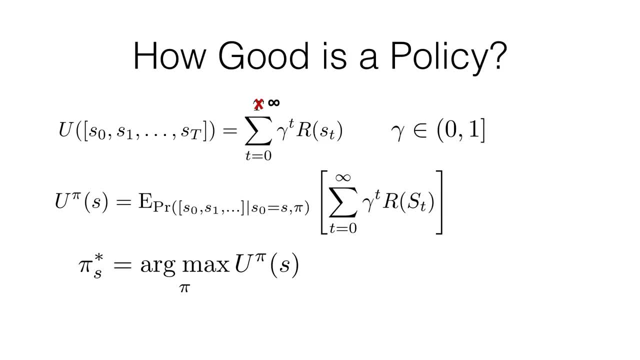 It has to suggest actions for every state on the board, every state in the environment. So what, for what reason, would just purely intuitively, forgetting about the math, imagine just, you know, one policy If you reach another state, if you reach state. 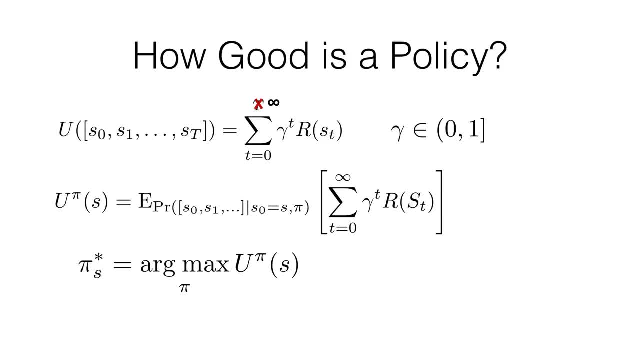 let's call it A. you reach state A. that policy tells you to take another action. It take let's, let's say: it tells you to move up from A And this is the optimal policy, right? This is the optimal policy starting from state S. 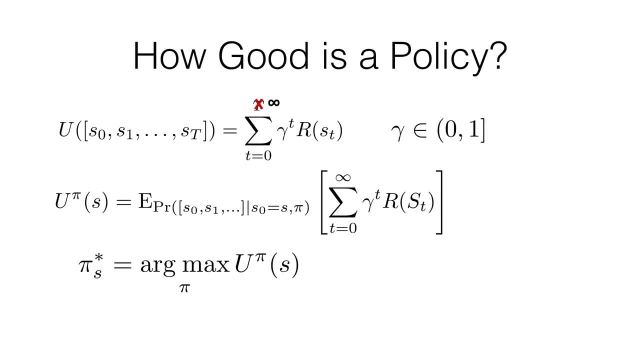 So if the optimal policy starting from state S tells you to take action up from state A, then there's some other policy. There's some other optimal policy starting from S prime. There's a different optimal policy and it also it also considers what to do when you're in state A. 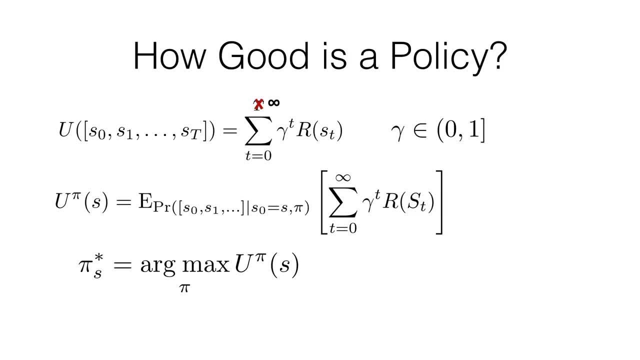 Why? why would it be a different action? Why would it not be up It? it would have to be up because that was the optimal move, right? If? if? if an agent using the original optimal policy ends up in state A, it has to move up and that's the optimal move for it. 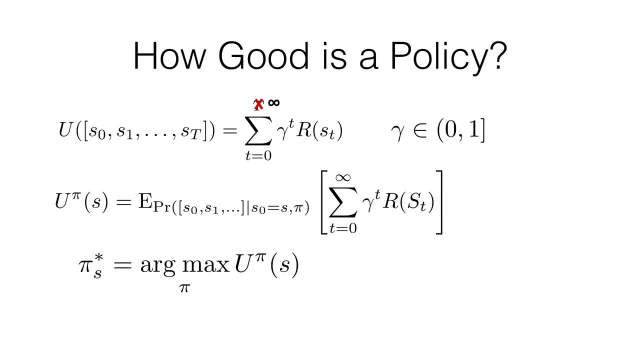 It doesn't matter where it came from previously, It just matters you know what its future reward is going to be. So the good- that's really good- news. That basically means that this initial start state that is part of our definition of the sequence score of the utilities. 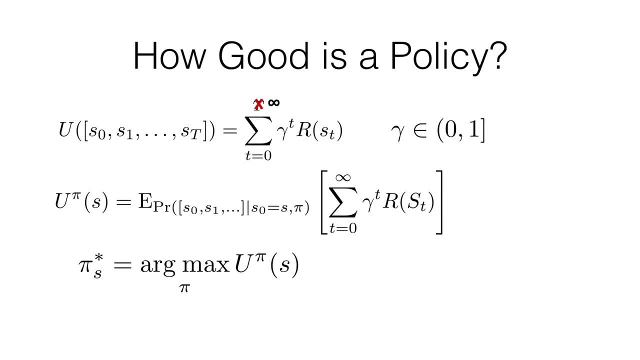 of sequences, that ends up being as part of the definition of the expected sequence score and and ended up, just by derivation, as part of the definition of the optimal policy. it basically can go away Because we can say: you know, it's the same policy. 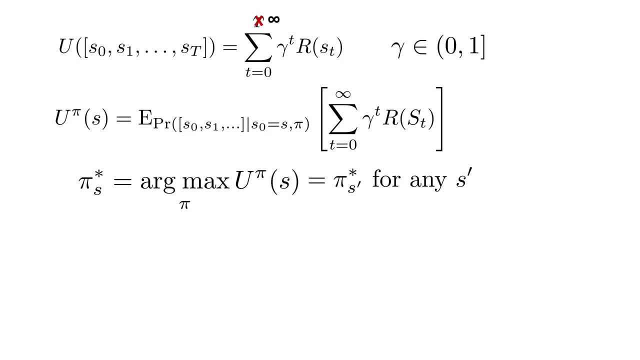 this policy is the optimal policy for state S, which also means this is the optimal policy for any other state S prime. So we can just drop the the S subscript. So we can just drop the the S subscript. So we can just drop the the S subscript. 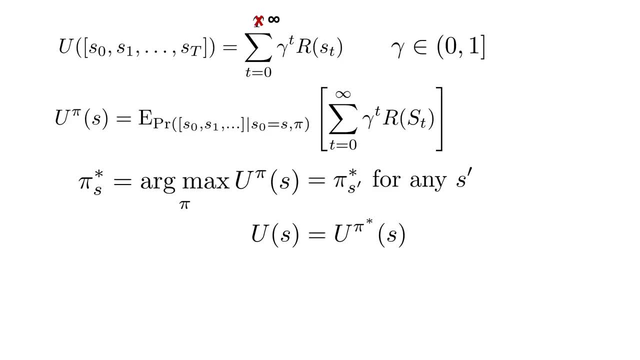 So then as a result, we can also drop some other notation to make things a little bit cleaner. We can just say: you know the utility for you know the optimal policy S is just, we're just going to call it the utility of S, right? 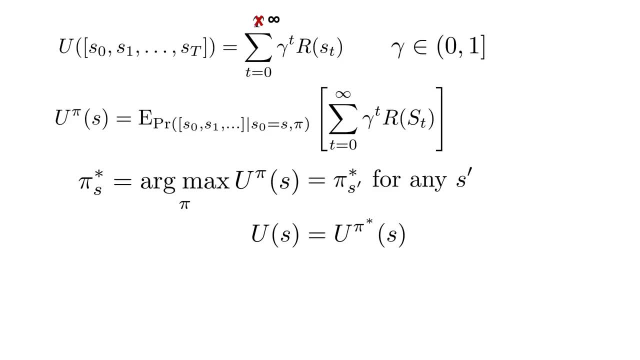 We're just going to say that the utility is implicitly defined to be the utility, assuming you're going to use the optimal policy from then, from there on, okay, And then the policy, The utility, can sort of be recursively defined by using this utility as saying that you know. 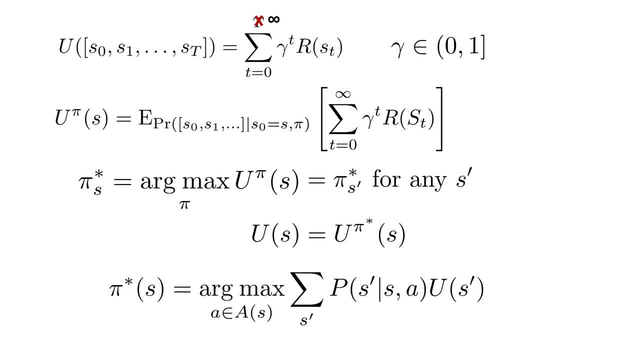 when we take the, when we are at state S, we're going to look at all the probabilities of the different transitions we can make given an action. or, more succinctly put, we're going to compute the expected utility where the utility has been defined by this. 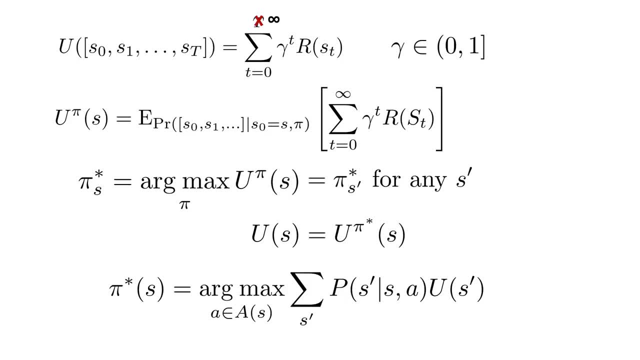 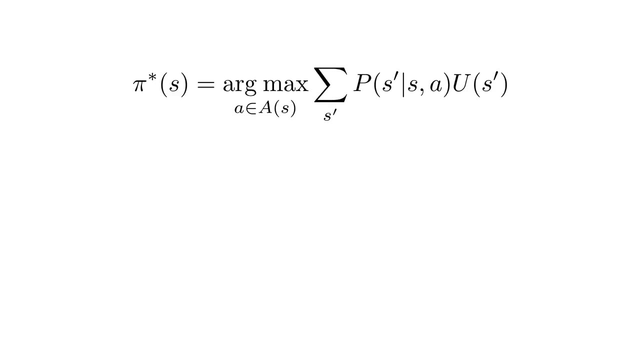 you know sort of optimality, this optimal strategy utility. We're going to take the expected utility, the probability of the states that we'll end up in if we take an action A and then we choose the best A. So this is all. this should all kind of start to look familiar. 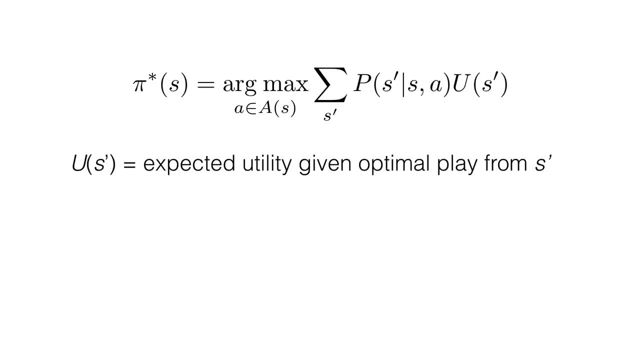 It was a little bit kind of a windy derivation, but the you know, the summary is that U of S, this utility score that we're really, that we're focusing a lot of attention on U of S or S prime in this case. 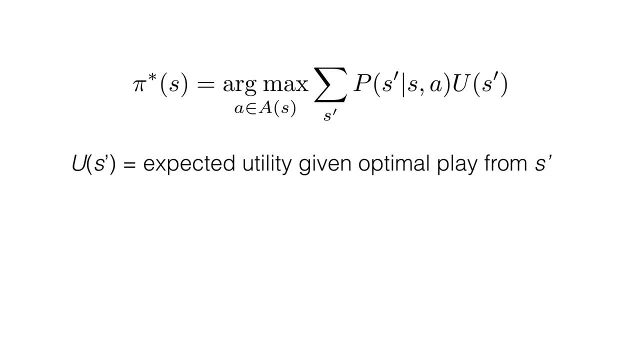 is the expected utility given optimal play from S prime right. Doesn't that sound familiar? It should, And and the idea is, you know, we don't necessarily know what optimal play is from S prime right. When we start, when we start to want, if we want to compute this policy, we start out with the idea that 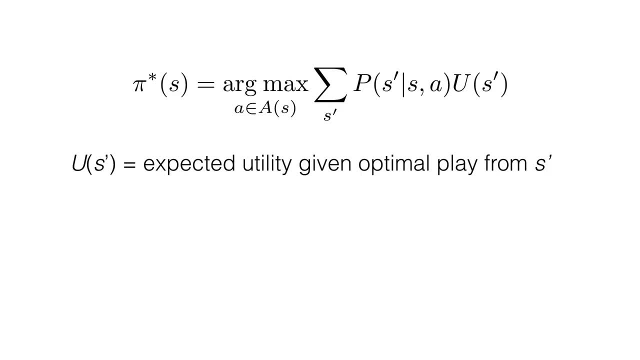 yeah, we. we know that we want to play optimally. we want to think about what happens if we play optimally. but we don't know how to play optimally. If we did, we'd be done. We wouldn't need to compute anything. 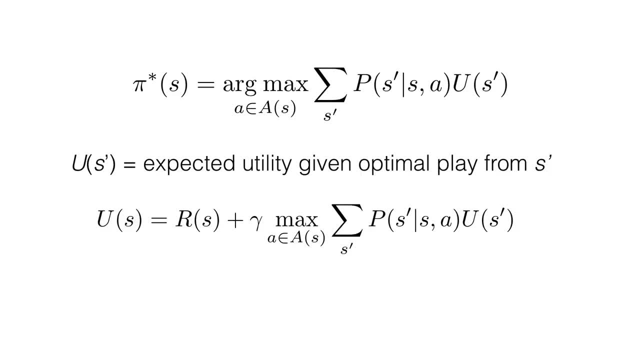 So you know, another way of writing this down is that the utility is the reward of the state plus the discount factor times the maximum expected utility moving forward. And this is, you know, this is a famous equation, this is called the Bellman equation, and you know. 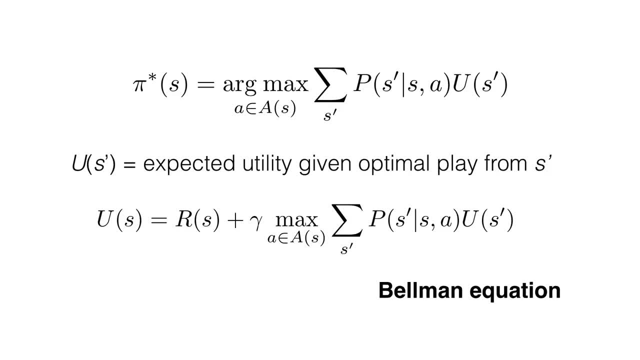 you probably have heard Bellman's name all over computer science education and he's he's inventor, one of the co-inventors of the Bellman-Ford, And you know he's done a lot of things, but this is one of his, one of his famous named equations. 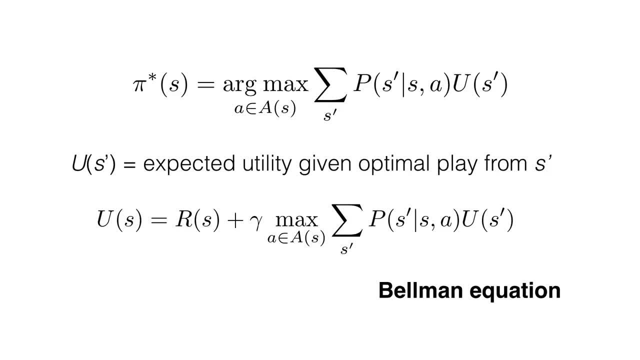 and it basically says that that this whole thing is very recursive, just like we've kind of seen before, is that, you know, the utility is the reward plus the future rewards and the utility is also all the future rewards. I mean it's kind of weird. so, okay, the utility is the expected future rewards for an infinite state. 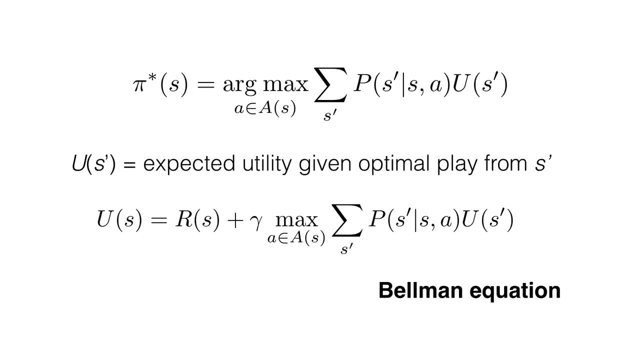 and it's sequence and that's defined with his recursion, because you can use the fact that you know if the utility is actually the future reward, expected future rewards, you can just use that for their neighboring states, for the states that you can, you can transition to, to compute it via this Bellman equation: 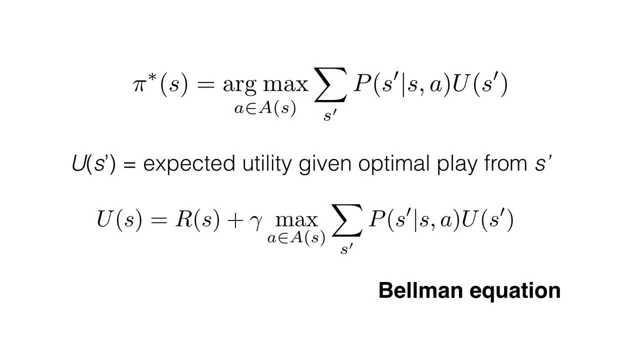 Okay, now how do we compute this? how do we use this to now find an optimal policy? And the trick is that we're not going to try to directly find an optimal policy, we're going to try to find these utility scores and then that will tell us the policy, or the policy we all 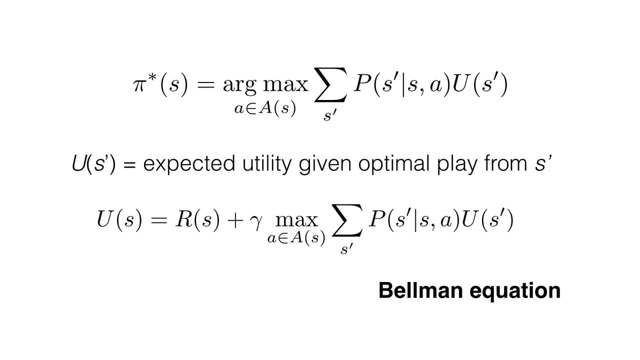 already saw on the last slide or even at the top here, it's pretty clear: the policy just looks at these utility scores. so the trick is now we need to compute these utility scores. okay, and it's. it's pretty weird because the algorithm to do this is, or the simplest algorithm to do this, is something called. 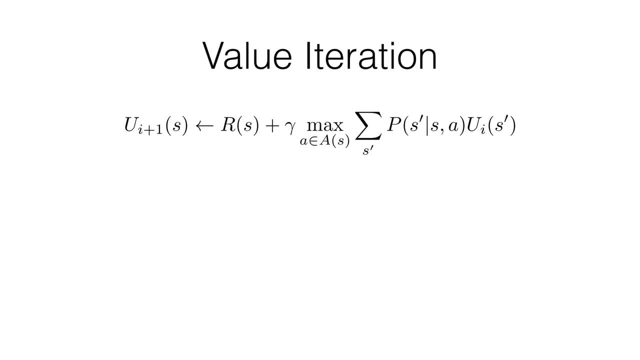 value iteration and it looks like this, which should look pretty familiar, because it looks almost exactly like what we just saw. this is: this is the Bellman equation on the bottom. the update on the top is the value iteration update. you know, and if you, just if you look at it and you see what I'm talking, 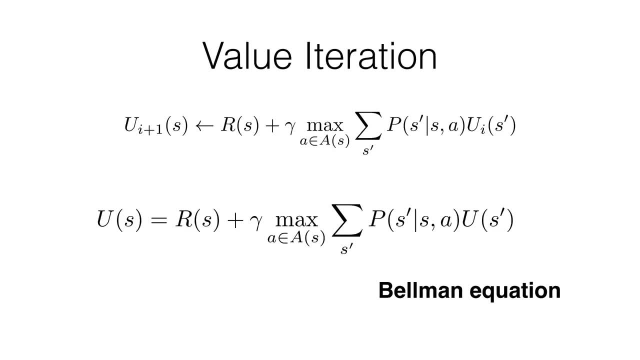 about why they look the same. they're. they're exactly the same, right, they are exactly the same thing. the only difference is that you know the value iteration version. you know it has the left arrow and notation to indicate that it's an assignment. so it's an algorithm. you're assigning the next version of. 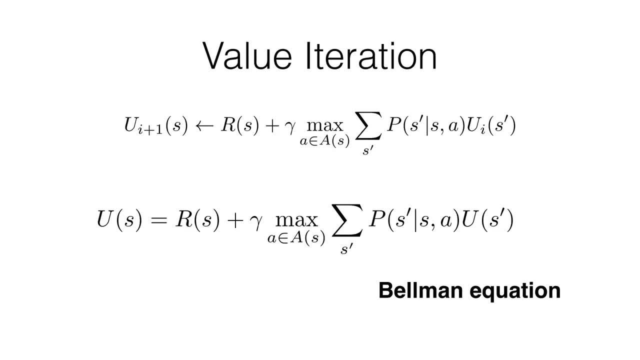 your utility score to be the definition of the. what would be the utility score if you know you of I. the current utility estimate was real and you can stare at this and think about you know why would this work? I mean, why would this work? basically, what it's saying is assume that your utilities are correct now. 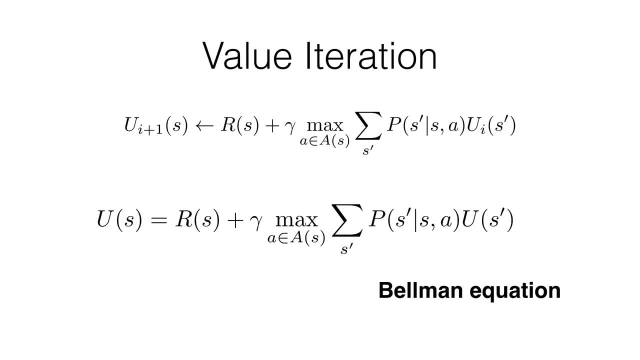 compute the utilities and for some reason, if you keep repeating this, your utilities in the end end up actually being correct, and you know that's a little bit weird. there's some, there's some math in the textbook that you can go through if you're interested in seeing the 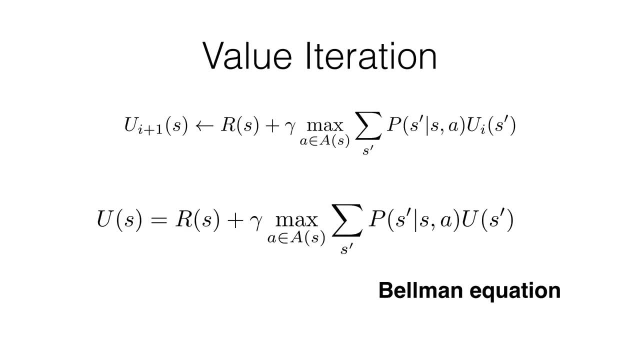 analysis of why this converges to an actual solution. but but it's actually useful, maybe, to think about. you know what happens? what happens with this update equation when it runs an update, and nothing happens. in other words, when it converges, when it's done so, what would, what would it mean for us to run? 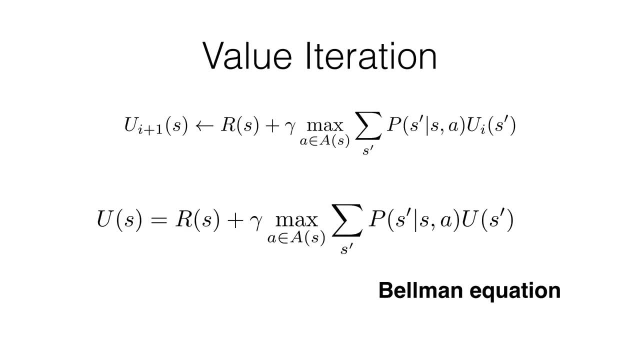 an update. you know upstairs the equation on top. if we run that update and nothing happens, right, you have a? u sub i plus 1 is exactly equal to u of i, u sub i, right. so if that, if that didn't change at all, what that basically means is exactly the. 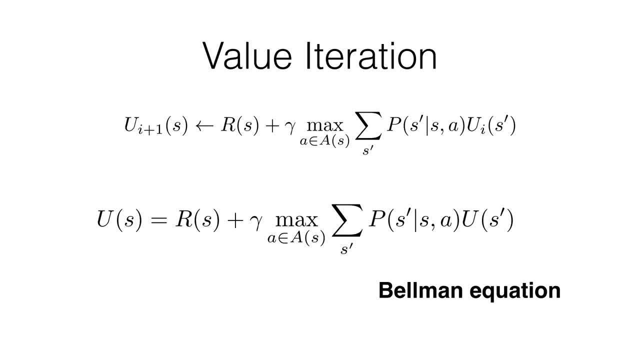 Bellman equation. it means the Bellman equation is is true, is satisfied, is correct. okay. and if that's, that's really good news, because that means that when we converge- assuming we converge- and you know, I defer the analysis of whether we actually do converge- but when we converge we will have satisfied the. 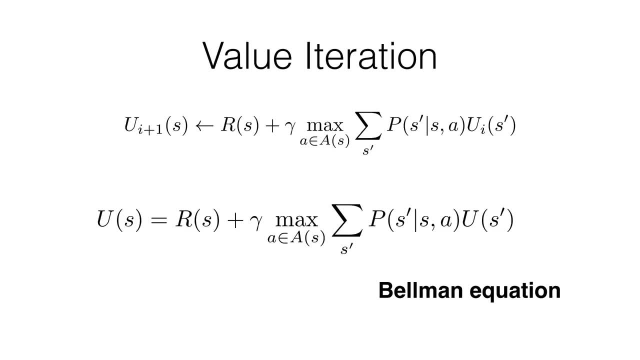 Bellman: equality, equality. okay, so let's run through an example of this, if it's a little bit weird, but it sort of makes sense. I mean, another thing you can think about is: you know, like I said, we've seen something like this before- the that max, that recursive max, inside this update equation is: is very similar. 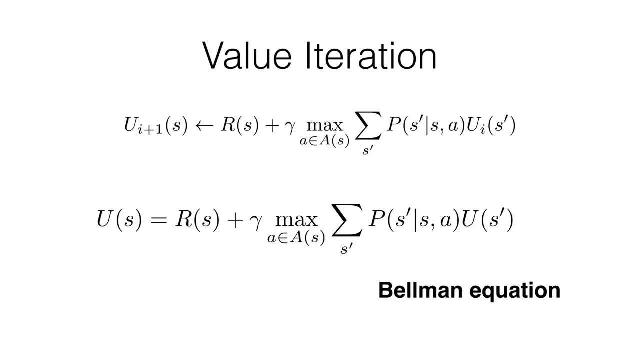 to. you know, minimax, basically right, or maxi max or expect a max. it's kind of the idea that let's assume, like we basically assume, that we're gonna do optimal later on and now we compute, you know, for our own decision. let's worry about our. 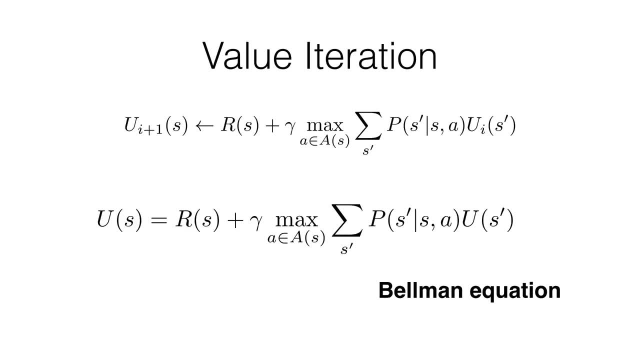 own our own problems, and our own problem is to maximize. assuming that the new u? u of i u sub i is telling us the truth, we need to make the best decision for our current decision, and then that iterates somehow and we end up at the solution. 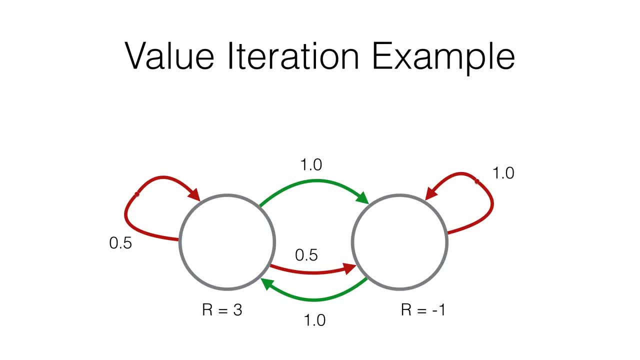 where it really is the true optimum. so let's let's run through an example. so here's a very, very simple markup decision process. there's two states, a left one in or right one, and the left state has a reward value of three, so that that clearly is the state we. 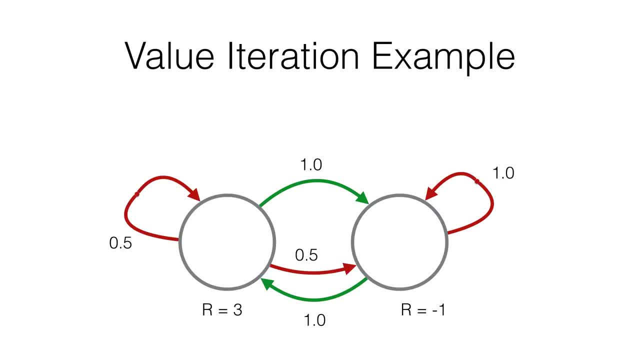 really like. the right state has a reward. reward value of minus one. okay, and the two actions that are available are red and green, so the red action is- I guess the analogy I was going for is that- the red action is you try to stay in place? ok, effort. entry into statement. •. and it understands that the option search over Darwin is a. then work on the curve leading to the target我问你: 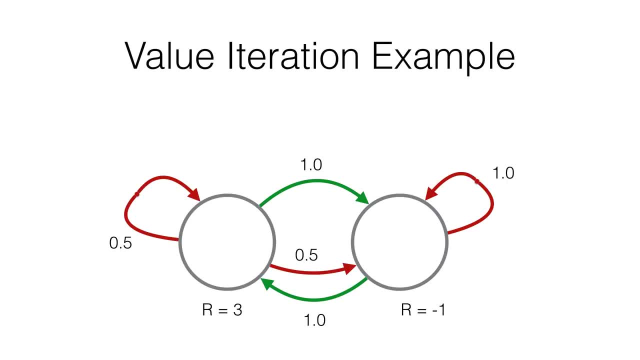 try to stay in place, you try to stop right, just like in a traffic light and a green action is: you try to move, you try to switch, you try to switch which state you're in and, in fact, if you look at the green, the green arrows, the green action, 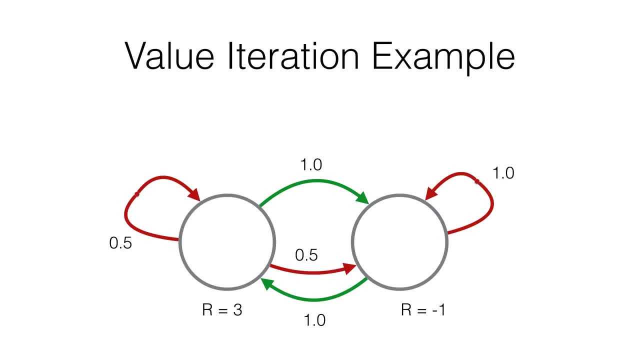 always succeeds right. it has a 1.0 probability of switching which state you're in. and then the red action. it succeeds when you're in the bad state. it succeeds in the right. so if you, if you're in the right, you can always stop and stay in the right and take more penalty if you really want to. but if 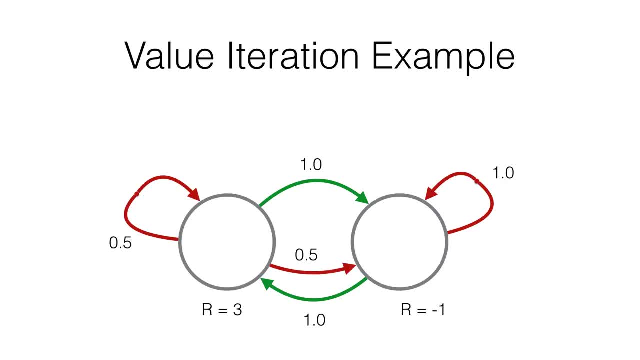 you're in the left. if you try to stop, you know there's a 50% probability you'll end up back in the bad state. okay, so this is clearly a very toy problem, but you can just imagine that this could represent something like: I don't know if. 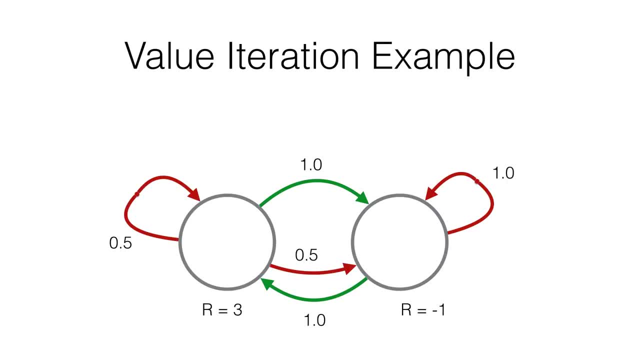 this actually works. but imagine you're trying to run a race and there's two modes. you can be in. you can either be in, you can be sprinting or you can be jogging, and maybe, if you wanted, if you try to stay jogging, you can always do. 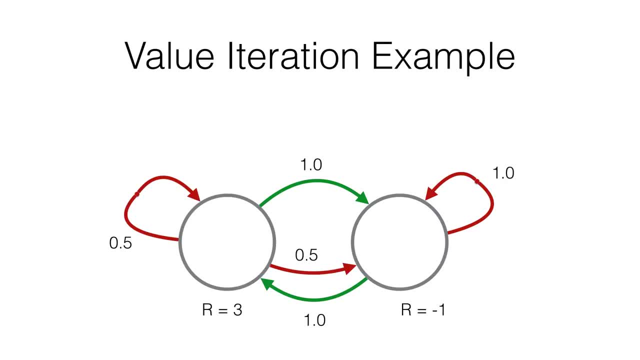 that. but if you try to sprint, if you try to, you can always start sprinting. but if you try to stay sprinting you get tired and you start jogging. I don't know, it's not the best analogy, but it's just the toy example with two states it's an easy. 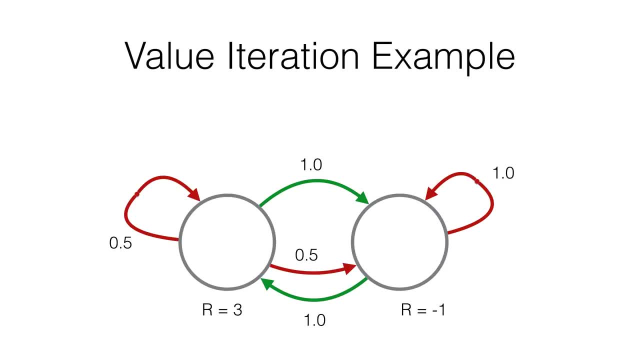 one to draw on the screen. it turns out that might have. decision processes are kind of hard to draw because you have to consider all the different actions. so I've color-coded here. but if I made this any more complicated it would be pretty hard to read. but let's start running, let's start trying to compute those. 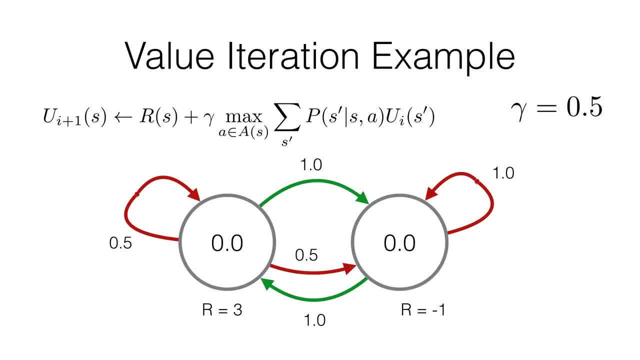 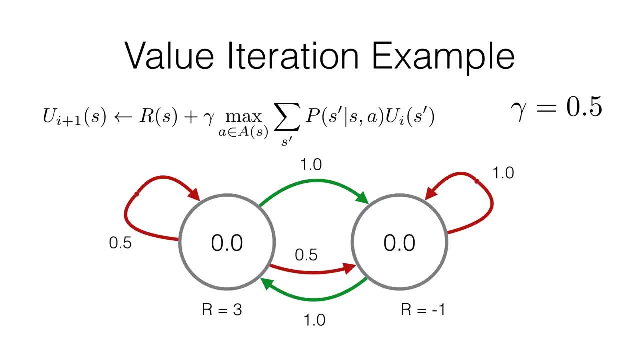 utility values, right, so so let's throw the data equation up on the screen. let's, just for the sake of this example, we'll say: gamma is point five. so so the. just for the sake of this example, we'll say: gamma is point five. so so the. 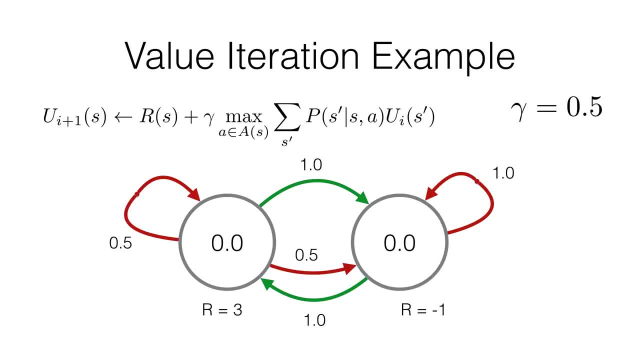 farther we go into the future, the is gonna- it's gonna- decay pretty fast. so that means that we sort of care about the next reward we get in the future about half as much as we care about the current reward. okay, and we start with utility scores of 0.0 as sort of as an arbitrary initialization. it turns out. 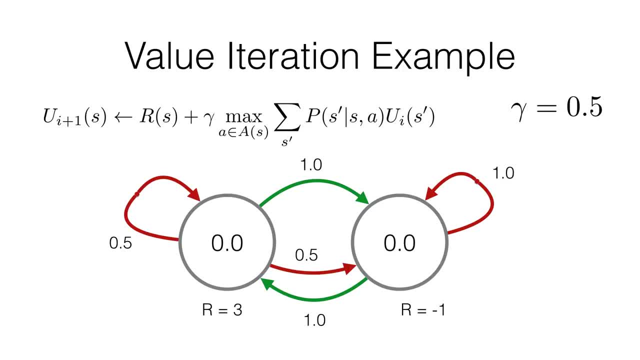 that it doesn't really matter when we give them these plus institutional really matter that much how you initialize, as long as it's not really really gigantic or or completely wrong, it sort of wants. you sort of want it to be on the same scale as the reward values, which are three and minus one. 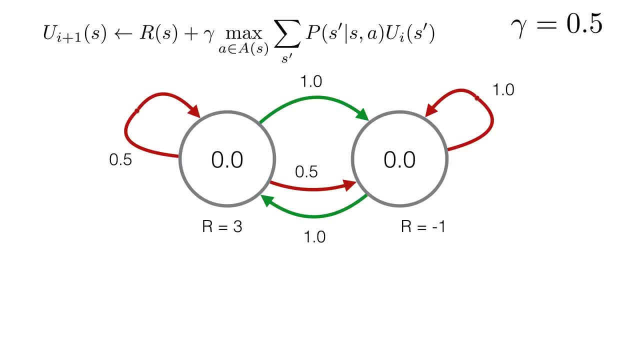 okay, but let's make some room. so let's start running these updates. so let's do the update for the left state first. so what is the utility for the left state? so we're gonna plug in the numbers and we get this. so we have, you know, R of s or R of left is three and you add 0.5, which is 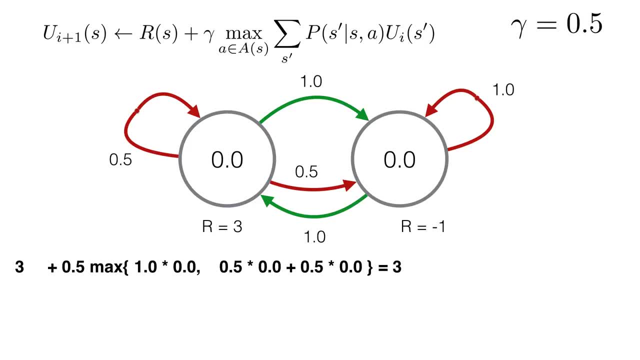 gamma times, the max of, you know, probability one of getting to the right state, but that utility is 0.0 and then probably point probability 0.5 of staying. that's 0.0 times plus probability 0.5 times 0.0. so all the 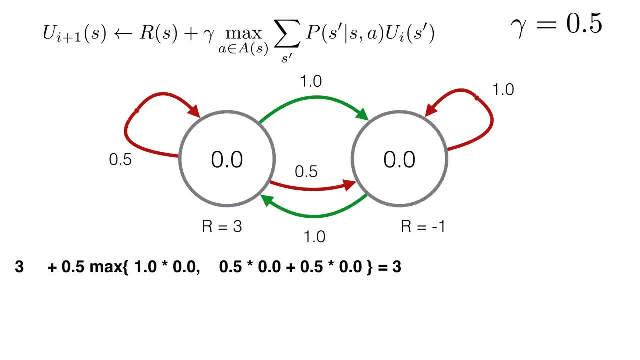 utilities inside that max function are just 0 right now. so we get 3, the answer is 3, okay, you, and then going, moving to the, the right state. we have the same, pretty much the same thing, right? so we have the, we have the reward of minus 1, and then we have 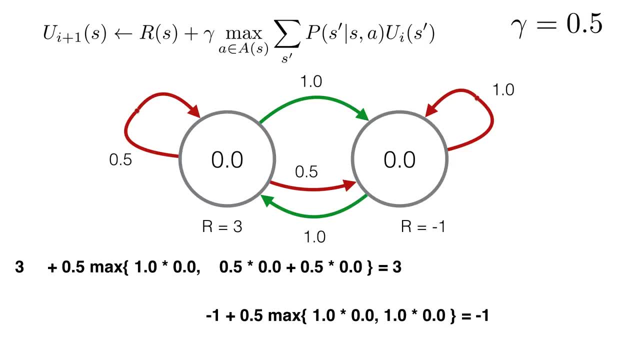 you know gamma times, basically 0, because our initial utilities are 0. so that was easy. so now our utilities are 3 and minus 1. okay, that's our current best estimate of the utilities, so let's continue updating. so on the left we have 3 again. the reward value just keeps popping in each of each update, you know. 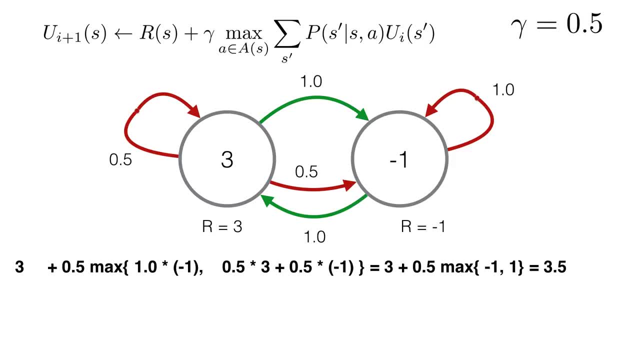 0.5, which is gamma times. now. now it's the max of you know one action, the green action, which is, you know, takes us with 1, 1.0 probability, to a state that we are currently estimating is worth minus 1. okay, that's, that means that you know the. 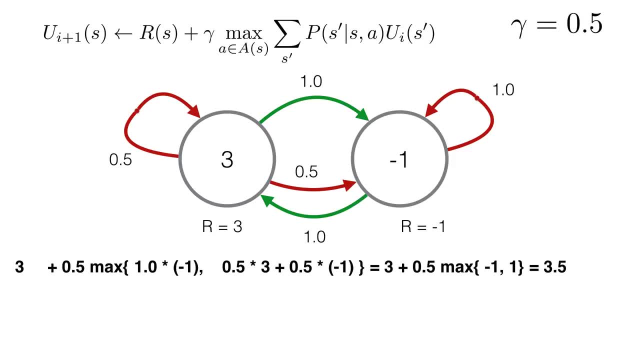 first option we have is to get minus 1 utility. okay, now the second option: we get 0.5 probability that we stay and we get 3 total reward there and then we get, and then 0.5 of probability we move to the right and get minus 1. so if you do, 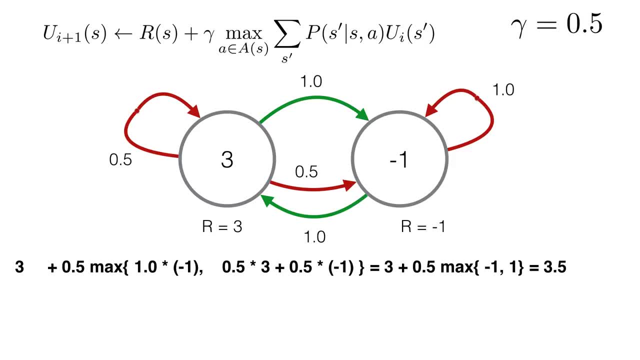 the math out, you get that we have a choice of getting minus 1 reward, expect minus 1 expected reward or 1.0 expected reward. so we want to take the max. so we get that the total estimated utility becomes 3.5. and on the right we can do. 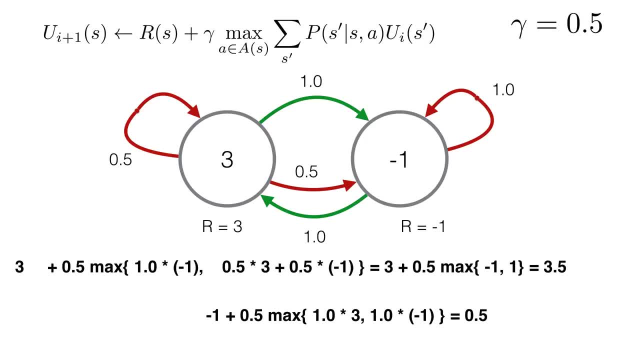 this again, you get, you know, minus 1- that's again the basic reward. the reward that's given to us by the utility is 3.5, and then we get minus 1- that's again the basic reward, the reward that's given to us by the environment- plus gamma times the max of 1.0, the 1.0 probability of moving. 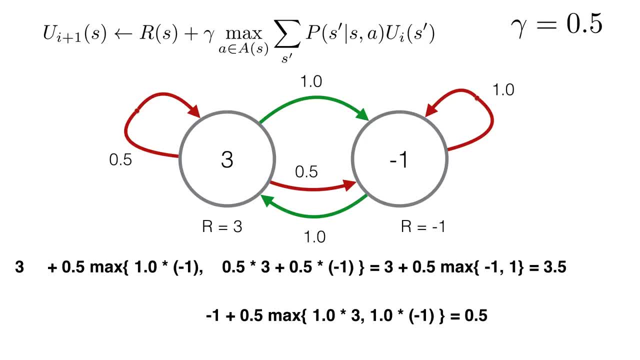 through the state that has a utility of, estimated utility of 3 and then a 1.0 probability of us, if we stay, of us getting minus 1. and of course we won't pick the minus 1 because we're trying to maximize. so we end up with a 0.5 score. 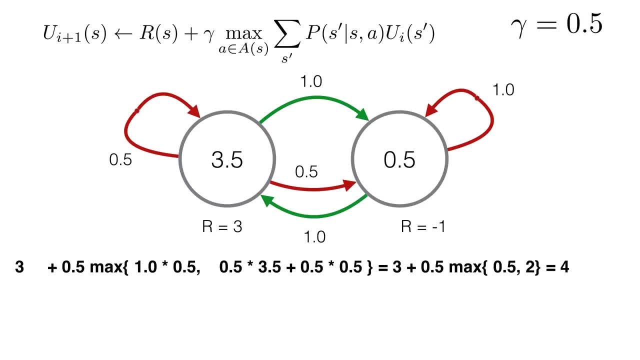 so we can run this a couple times more. you know, if you want, you can probably, you know, pause the video or something and check the math. but it's basically arithmetic at this point and you know you can see the, the numbers sort of converge a bit. so so actually, let me let me back up, so it would be useful. 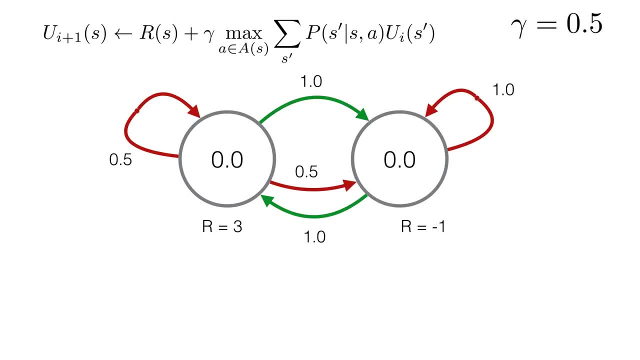 to see this from the beginning. so, if you see, from starting from the beginning, let's just watch the numbers now. so forget about the equations, forget about the equations that are gonna pop on the screen. I'm gonna just cycle through these slides so, you see, we get, you know, 3 minus 1, and now we get 3.5 and 0.5, and 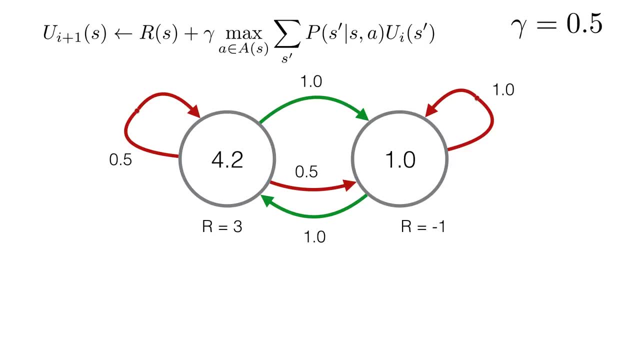 we get 4.0 and 0.75, and you get 4.2 and 1.0, and we get 4.3 and 1.1 and 4.4 and 1.2. and I didn't do all these by hand. I actually computed some of these with some code, just cuz. 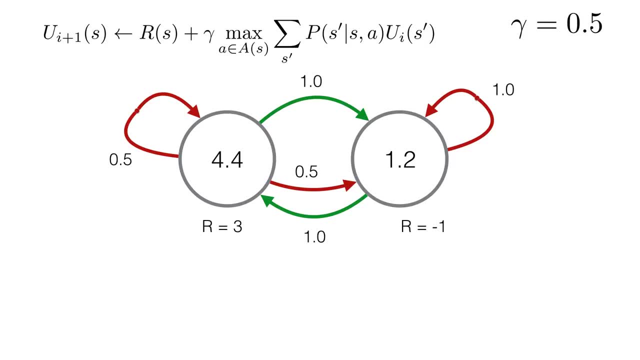 even though this is a tiny example. I got pretty bored doing these by hand. but here's the interesting part: this is where it converges. it actually converges to these the the previous slides I was rounding. this is not rounded. this is the actual numbers, so it's 4.4 0 0, 0, 0 0 and 1.2. 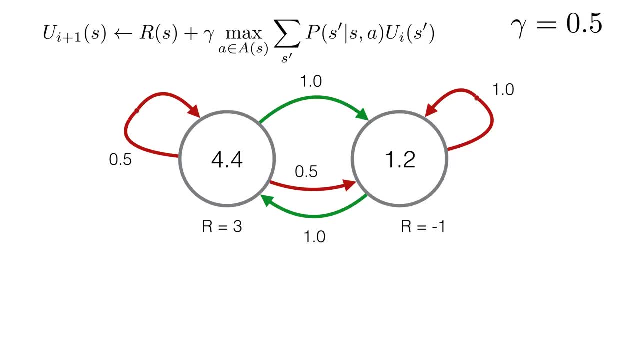 0 0 0 0 0. okay, so this is the actual converged utility value for this example I drew on the screen. so that's great, I guess. I mean it's not really that exciting because these are just random numbers, we're not arbitrary numbers. but 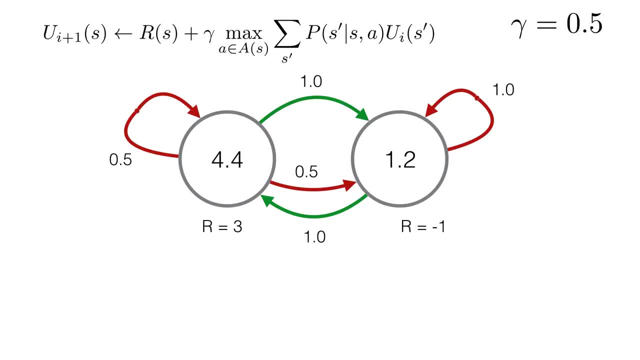 one question that's kind of interesting to ask is: did you know this really work? this is: did this really converge? well, let's think about it. so how can we check that? we can check that by plugging them, these numbers, into the Bellman equation. and so what happens if I plug those numbers into a certain equation? so let's 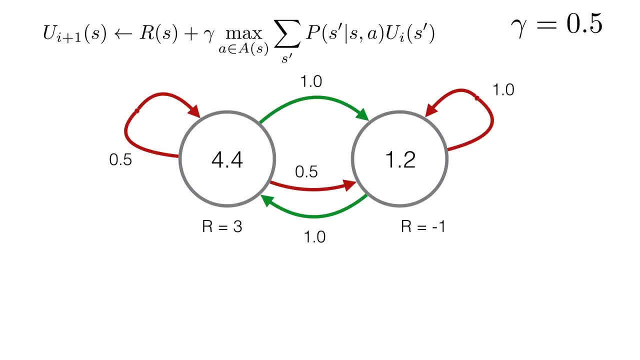 do that. so when we plug in the numbers, we have that you know, the number we're going to be looking for is, you know, 3, the reward plus gamma, which is 0.5 times the max of, you know, 1.0 transition probability to get to the state that we. 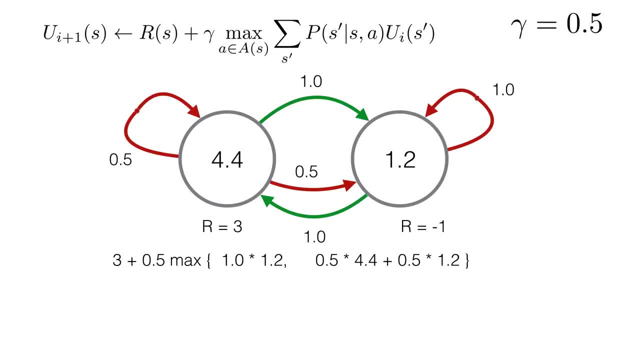 have estimated to have a utility of 1.2, right, so that's 1.0 times 1.2, then 0.5 probability of us staying in the 4.4 utility state and 0.5 probability that we end up in the 1.2. okay, and if we do the arithmetic we just get that, you know. 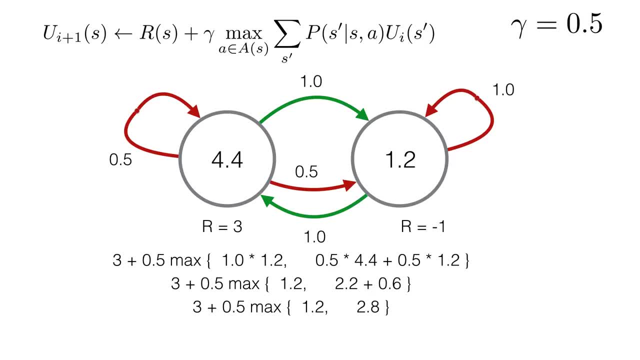 that's either 1.2 or 2.2 plus 0.6, okay, and then finally, you do the math out fully. you're going to pick that, you're gonna pick the 2.8, not the 1.2, and so you end up with 4.4. okay, but that's good right, because 4.4 is the value, is the. 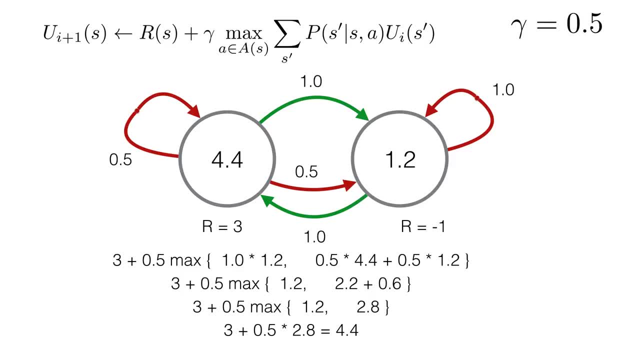 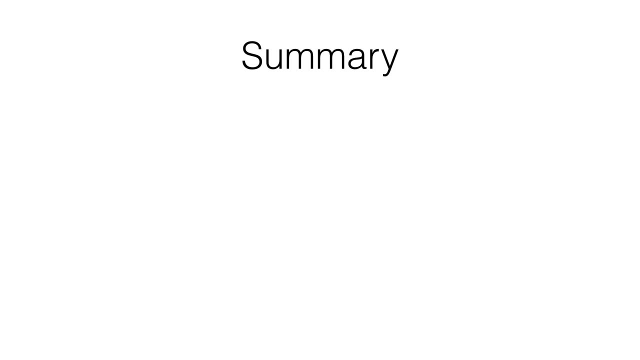 value we want. so this means that that that recursive definition is actually true, is actually true, is actually true, is actually, you know, finally true for these, for these values of you, right, these values of the utility function. okay, so that's pretty much it. so, to summarize, we talked. 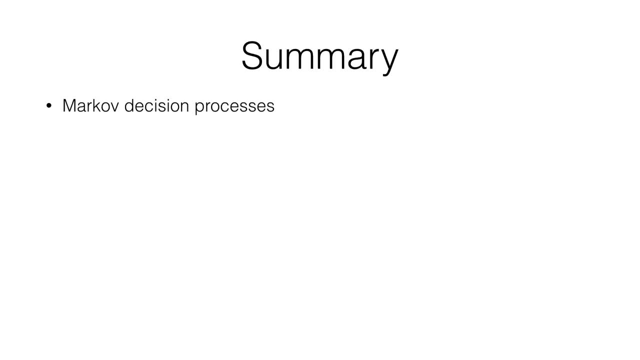 about Markov decision processes and, and if this is again so, it's important to separate the, the state representation or the environment representation, from the algorithm for doing AI in the environment. so a Markov decision process is not. it sounds like it's a smart AI representation or something. all it is is an environment. it's a dumb environment. 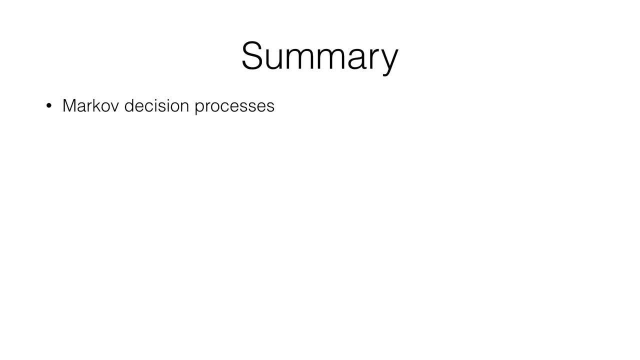 it doesn't. it doesn't do anything smart, it doesn't do anything rational, it's just. this is a place that we can stick our AI agent and the AI agent can try to do something smart in, but it is just an environment. it's the maze for the rat. 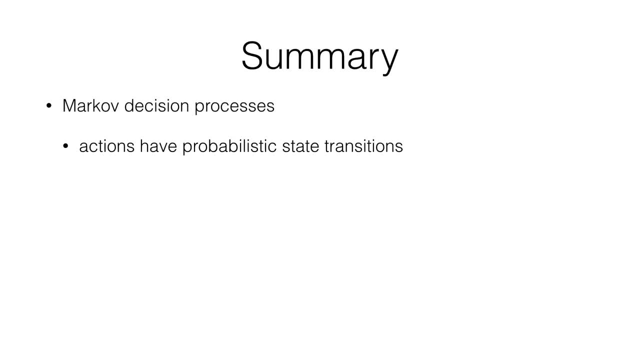 okay, so the markup decision process is in. you know the maze, where, where the actions now have probabilistic state transitions. that means that the agent, the rat in the maze, gets to choose an action and when it chooses an action, the maze determines where the the agent ends up, where the the rat ends up after choosing to move one direction. okay, the rat. 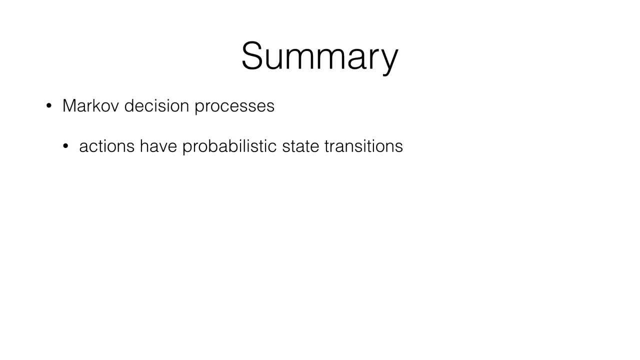 analogy is not working as well anymore, but the point is that the, the agent, chooses the action, but the markov decision process takes that action as input and determines where, what state the agent ends up in. okay, and and to start to think about making rational decisions in markov decision. 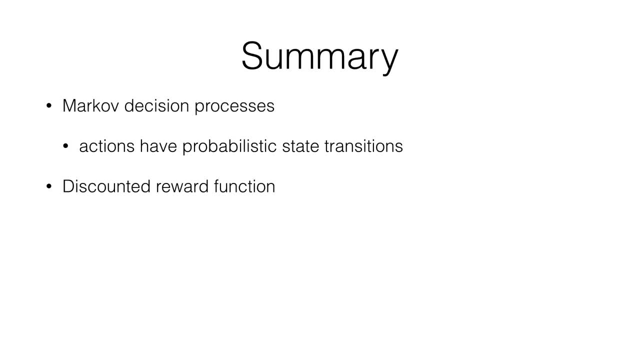 processes. we came, we came up with a definition of a discounted reward function that enables us to think about future rewards even in infinite time series. right, even if we say this agent's going to wander around the state space until infinity, until eternity, we can still think about you know, we can. 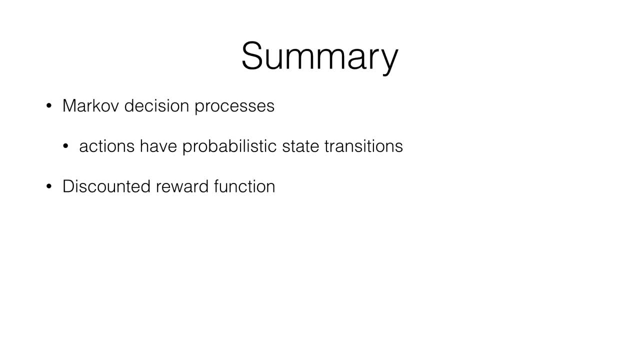 still think about that with finite numbers. so the discount reward function just sort of waits the future rewards less. and we talked about the notion of what an optimal policy does. an optimal policy is going to maximize the expected reward or the expected discounted reward, and you know, in wrapped 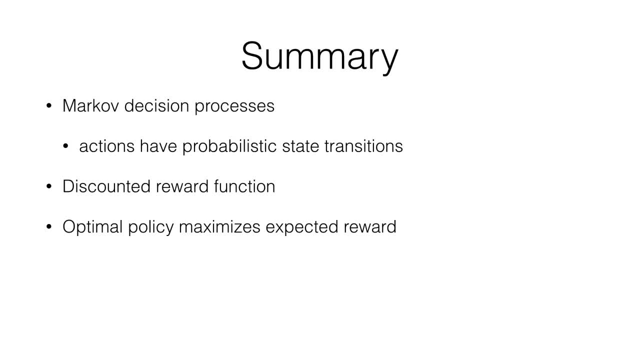 up into those. we talked about the definition of a policy, which is just a function that takes a state and tells you what action to do, and finally we got to an algorithm that can compute an optimal policy, called out a value iteration. okay, and this is just. it, basically just. 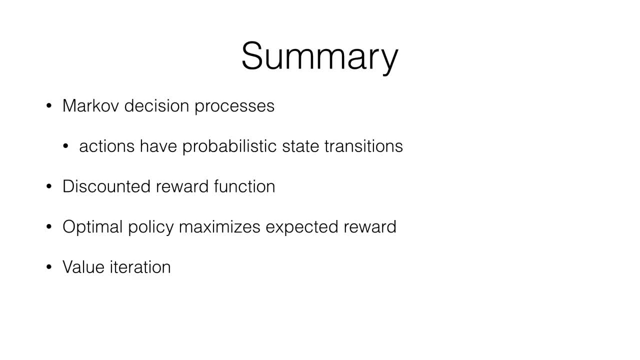 computes the values, assuming it knows the values of every state, it updates values based on its assumed values and eventually that converges to the point where the updated values and the assumed values are the same number and that you can show with some math and some thinking, or maybe. 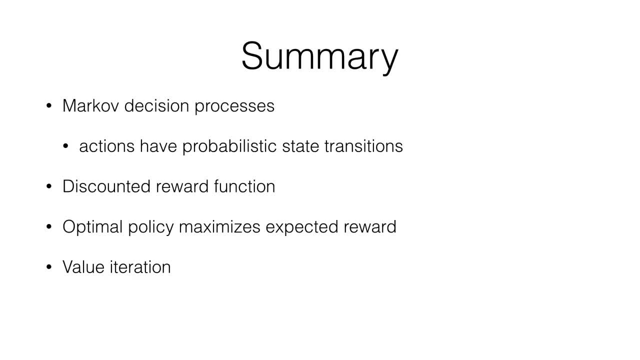 just if you want to trust me that that is actually the optimal, the optimal value, okay, and the material was uninvolved. be careful you even use in a davenportameter, whatever. it is a matter of fact. that's not to say you can't get stuff done I. that's not to say that. it's not to say it's industries are there. it's very anything. 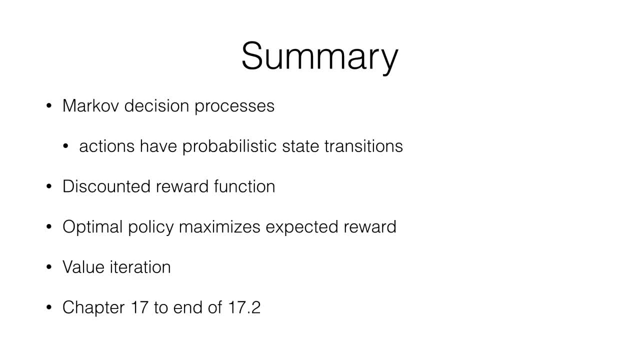 And the material for this stuff is in the textbook in Chapter 17, and it goes until the end of Chapter 17.2 or Section 17.2.. And we'll get on to the later stuff later, so you can read ahead if you want.